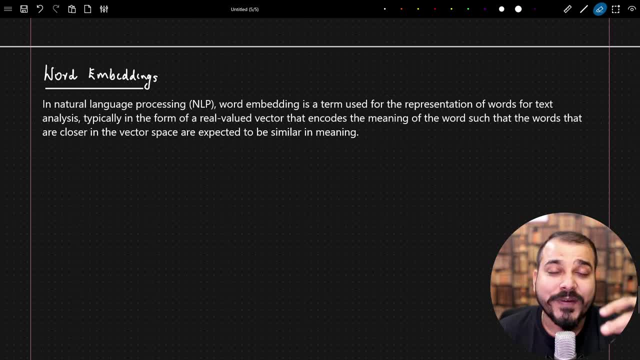 keeping this particular topic at this point of time. Why? Because we have discussed so many topics wherein we focused on converting word into vectors. So now you'll be getting a very clear idea about what exactly word embeddings is, and here I've given you a Wikipedia definition. So 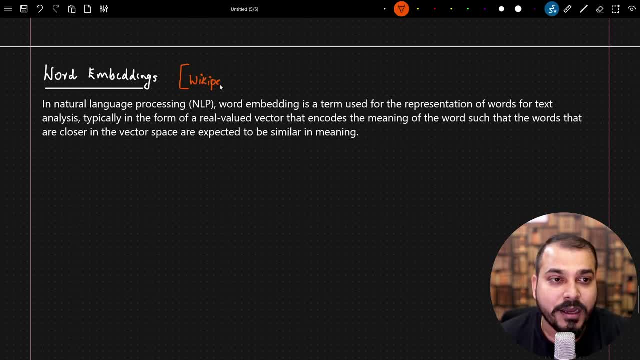 this is a very simple Wikipedia definition. I have taken it from Wikipedia, So the entire credit goes to Wikipedia over here. So over here you can see the definition that in natural language, processing word embedding is a term used for representation of the words right For text. 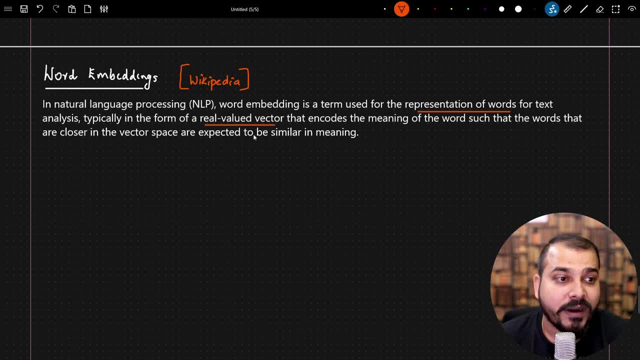 analysis, typically in the form of real valued vectors. that encodes the meaning of the word, such that the word are closer in the vector to the word. So this is a very simple definition. So let's say that I have two words, king and queen. okay, Or forget about king and queen. Let's say 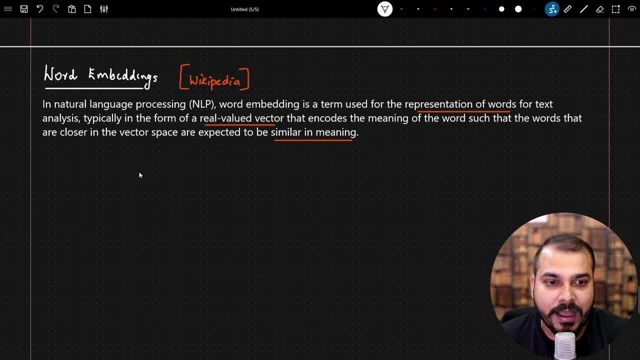 that I have two words, and the two word is like happy and excited. right, Let's say, I have this two specific word. Now, when I have this two specific word, with the help of word embedding techniques, what we do is that we convert this particular word into vectors. So let's say that: 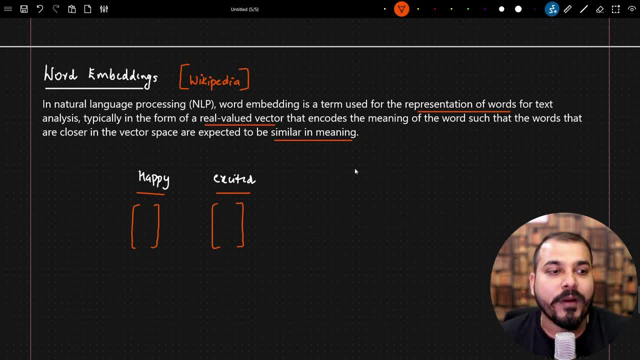 I have two vectors and let's say, if I try to plot this vectors in a two-dimensional graph, okay, And if I really want to convert this into two-dimensional graph, we have techniques like PCA or other techniques, which is an unsupervised technique to do dimensionality deduction. So once, 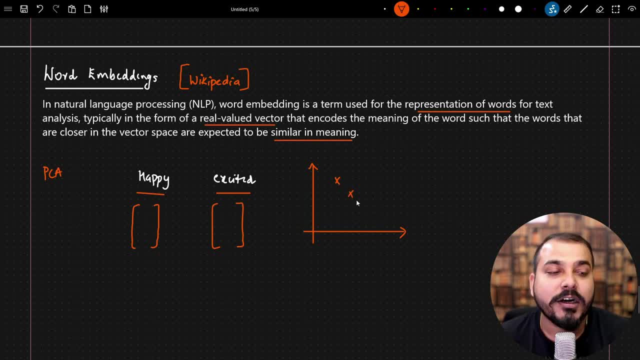 I probably plot this. let's say: happy and excited are coming near to each other Based on this particular vectors. it basically indicates both are similar word. okay, Let's say that I have one more word like angry and excited. So let's say that I have one more word like angry and excited. So 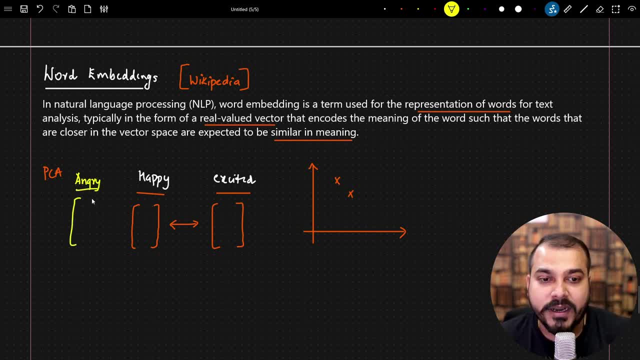 let's say that I have one more word likeパパ, which is one of the conglomerate trial. 이� procedence and all imprison effort of one word is equal to two words like aggr, rry, right. And then, in this case, with the help of word embeddings, if I am trying to convert these into vectors, the tentative. 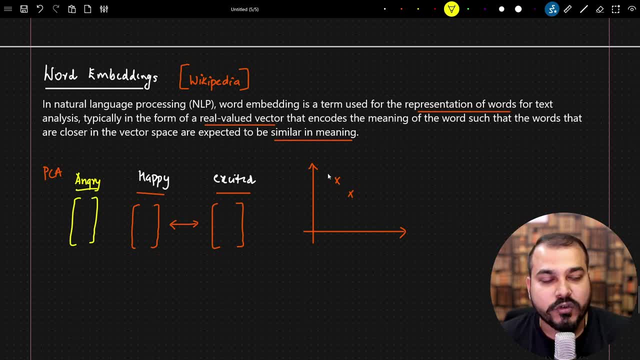 thing is that obviously happy is the opposite to angry, so angry will be somewhere here, if I probably try to plot this particular vectors over here, why? Why it is coming so far? because it is an opposite word. So the distance between this world will be quite high, whereas the distance 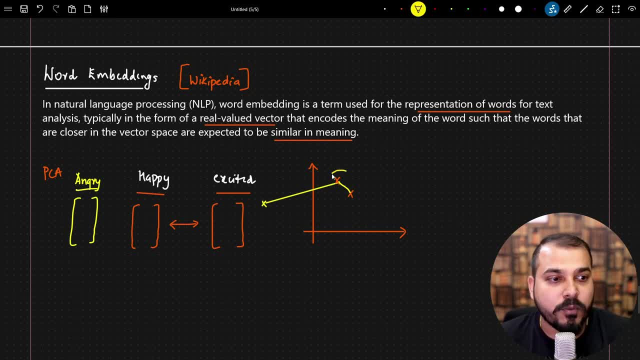 between this particular word will be quite less. So this indicates that this- both the words are similar, whereas this- both words areボ, styles and Run etc. is indeed similar. For that reason I would not attempt this as either squared or quadrupled and you would not expect thisrakable. 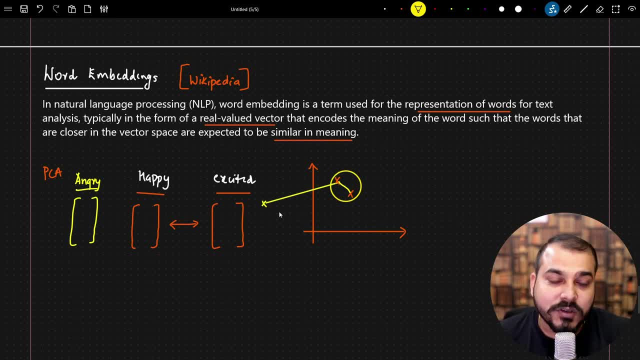 Whereas this, both words are opposite to each other, right, And this is all possible because of efficient conversion of the word into vectors, right, And how we are doing this, again with the help of word embeddings, but the techniques we have learned till now is it is something like one hot encoded. 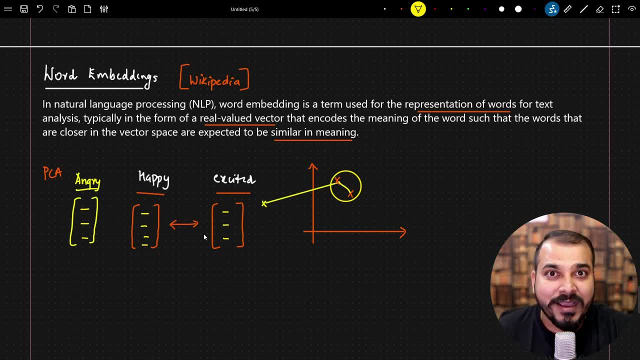 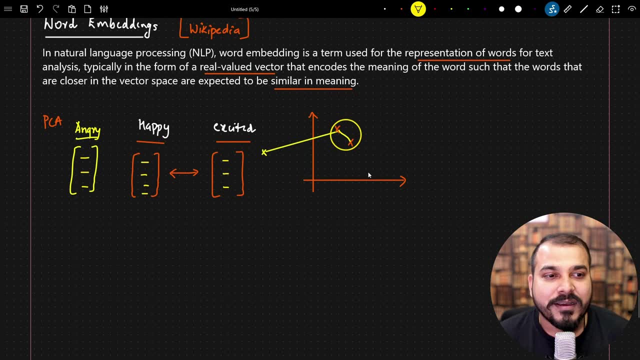 We have learned about bag of words, We have learned, TFIDF we have learned, and all these techniques are a part of word embeddings. So if I properly clearly show you the division, you know in the first step, if I have the 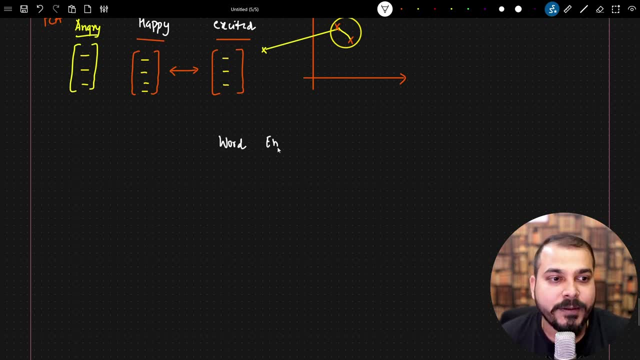 word embedding techniques. so let me just again go ahead and write it. Word embedding techniques are specifically of two types. So this is my first type and this is my second type. The first type is based on count or frequency. count or frequency. 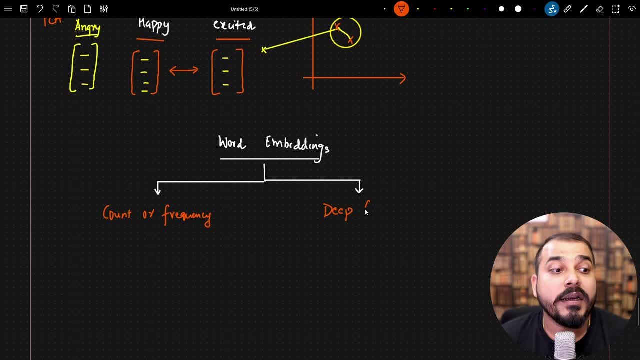 And the second type is based on Deep learning, trained models. Please hear to this very properly, because this deep learning, trained models will give you very good accuracies. Okay, Now, in count of frequency. we have learned about three different types. One is one: hot encoded. 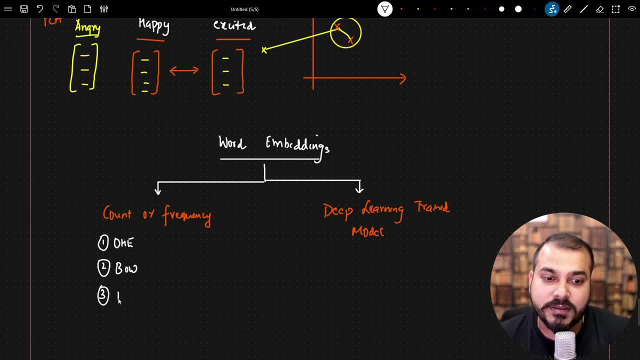 Second one is something called as bag of words And the third one is something called as TFIDF, right. So all these techniques we have learned right And we know the advantages and disadvantages. We are focusing more on count of frequency, right. 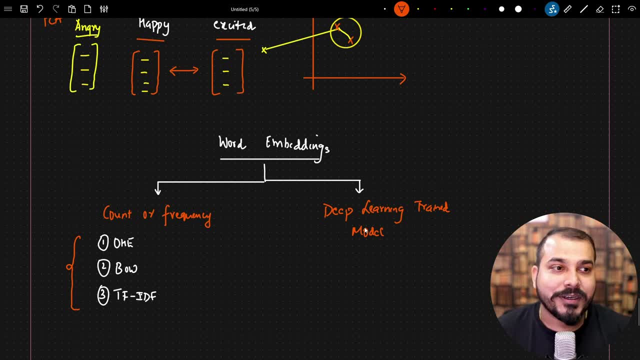 But the major one, which is having a better accuracy, which is actually- and all these techniques, at the end of the day, is also converting words into vectors, or it is converting sentence into vectors, right, Sentence into vectors. But we have seen a lot of advantages and disadvantages. maximum number of disadvantages are there. 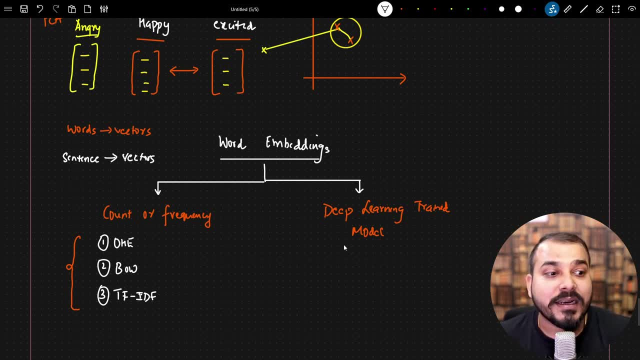 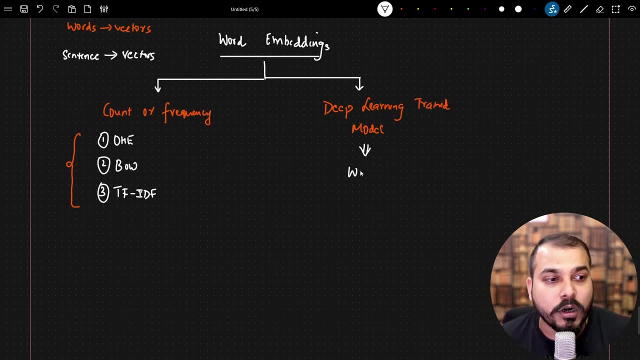 with respect to all these techniques And this. all disadvantages are getting solved by this deep learning. Deep learning, trained model, And the trained model is nothing but which is basically called as word2vec. It's not like we cannot create it from scratch. 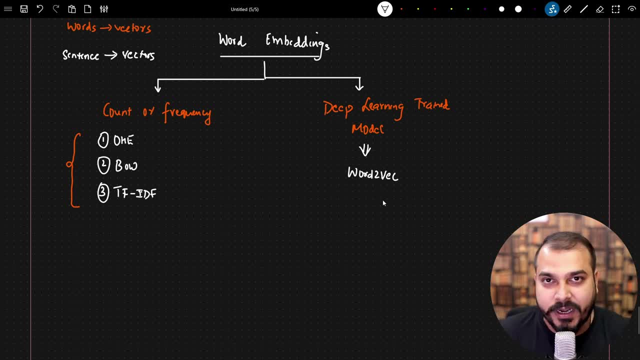 We can definitely create it from scratch, but again, you require a huge amount of data. And what we are going to do in that. first of all, we are going to understand in the upcoming videos what is exactly word2vec and how it is basically converting a word. 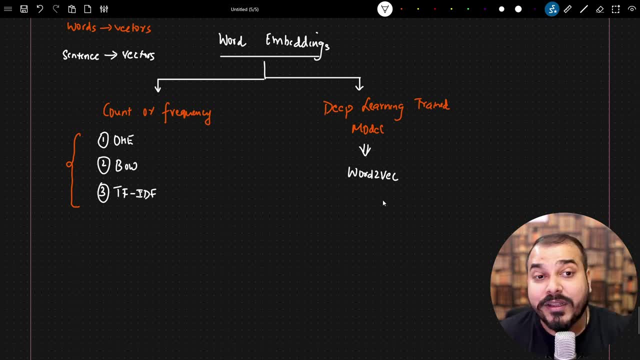 into vectors and how it is solving all the disadvantage things that were there in this particular technique, Everything we are going to discuss. But just understand that what is word2vec? It is a word embedding technique which will efficiently convert a word into a vectors. 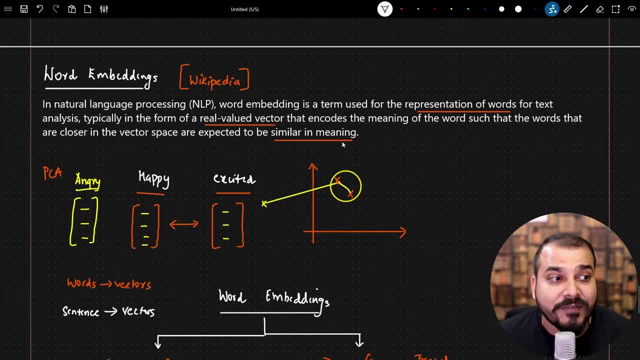 which will be making sure that both this property it is expected to have similar in meaning whenever it is converting into a vector space. Along with that, it will also give you a very good representation of the words right Sparsity will not be there and all. there are many points which I'm going to discuss. 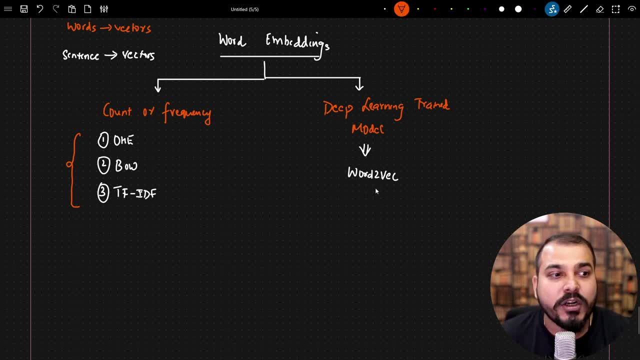 in the upcoming videos with respect to word2vec. Now, word2vec are of two types. One is because the entire deep learning architecture is built on word2vec. Now, word2vec are of two types. One is because the entire deep learning architecture is built on word2vec. 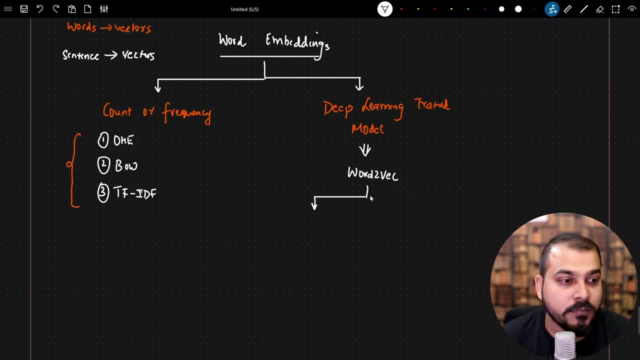 Two different types. One is we basically say cbow, C, bow, Cbow is nothing but continuous bag of words, Super important continuous bag of words, And we are also going to see that, how the models get strain. But for this you really need to have a prerequisite: knowledge of how an ANN works. what is loss? 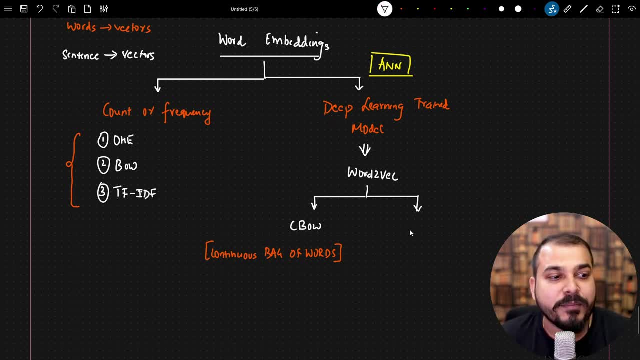 function, What is optimizers? and all right. The second technique is something called a skip gram, skip gram. Again, this is a different technique And again it is a part of word2vec itself. It is a different type of word2vec. 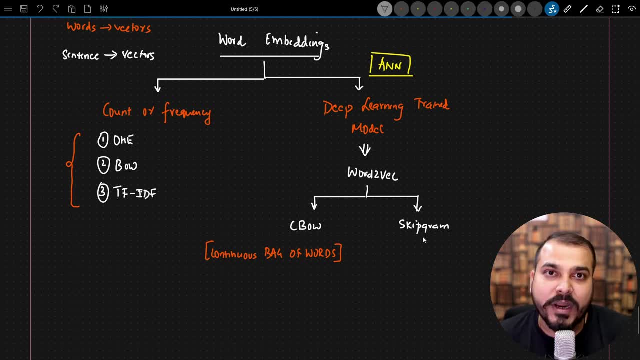 At the end of the day, we can either use CBOE or skip gram to get an efficient conversion of word2vectors right, And this is what we are going to see. We are also going to see some pre-trained models of word2vec, you know, probably created by Google. 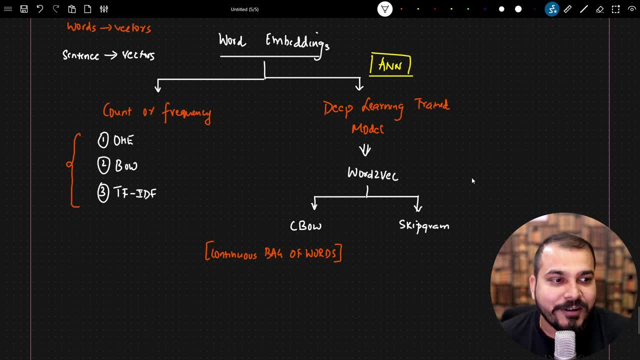 and it is somewhere around 1.5 GB big model size. We'll try to download it, We'll try to see, we'll try to execute it. But in the upcoming videos what we are going to see is that how word2vec word embedding, works right. 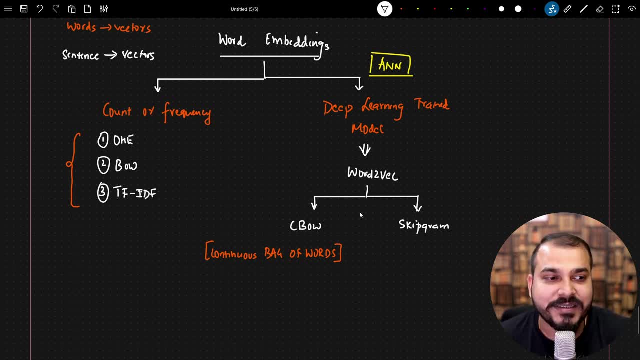 And how it is making sure that all these disadvantages that are present in these techniques is getting removed. Right, So this is what we are going to discuss, but I hope you got an idea At the end of the day, whatever techniques we have discussed till now in converting word into vectors. 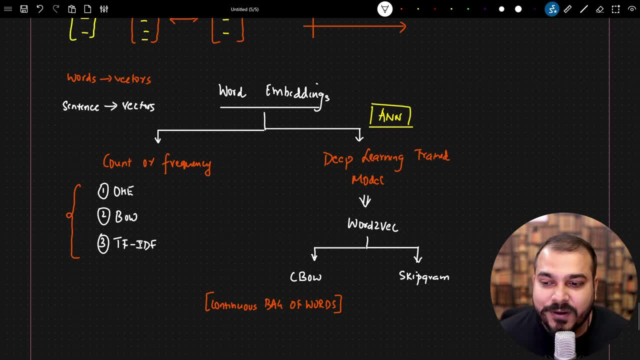 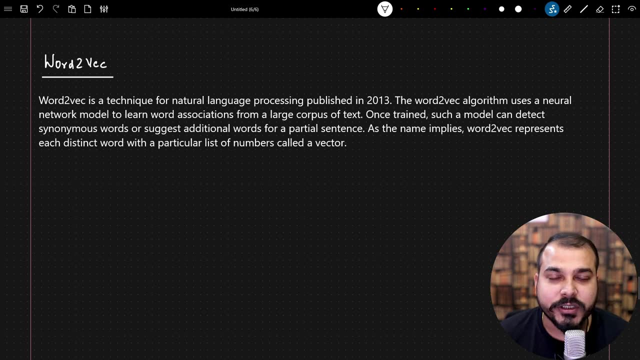 it falls under word embeddings, right? So, yes, this was it from my side. I will see you all in the next video, And in the next video I'm going to discuss about word2vec. Hello guys, So we are going to continue our discussion. 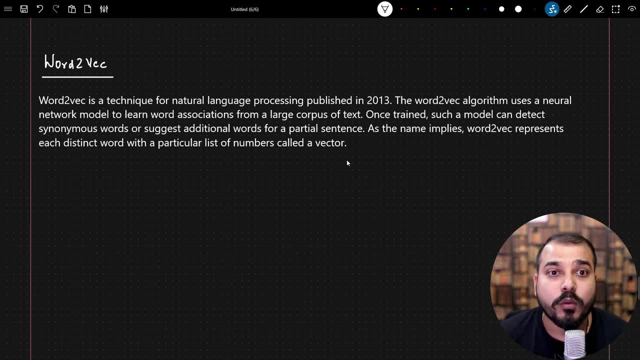 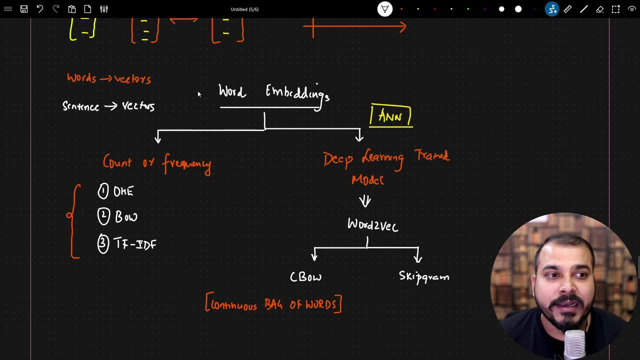 with respect to natural language processing. In this video we are going to cover word2vec. We have already seen what exactly word2vec is. It is a deep learning trained model And again it is a kind of a word embedding techniques. 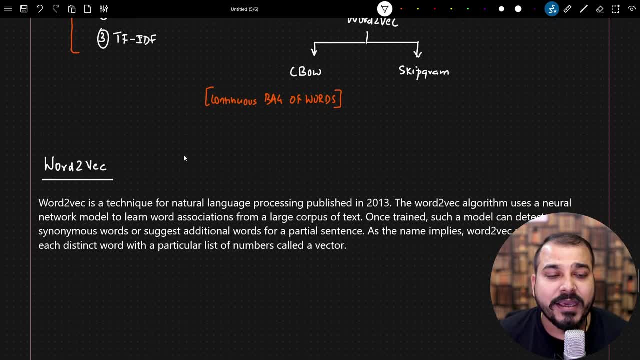 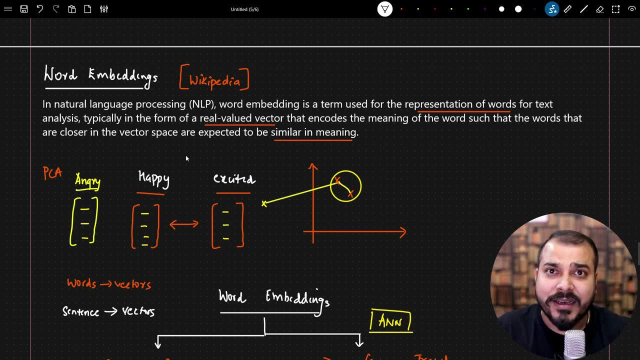 wherein the focus is to convert word into vectors, making sure that the meaning of different, different words are actually maintained, Like if there are similar words. we'll be getting vectors that are very near to each other, If we'd probably find out a difference, and we'll also be able to see that. 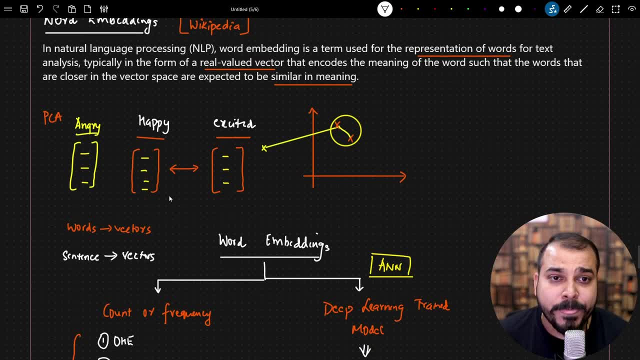 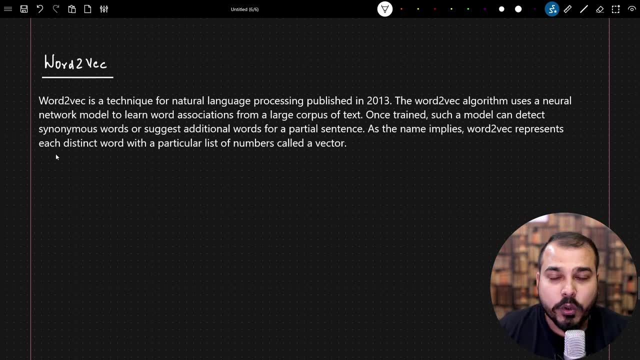 which all words are completely opposite, based on these vectors. okay, So let's discuss about word2vec And I will give you an idea about, like, what exactly is word2vec and how the words is getting converted into a vectors. In the upcoming videos I will try to show you. 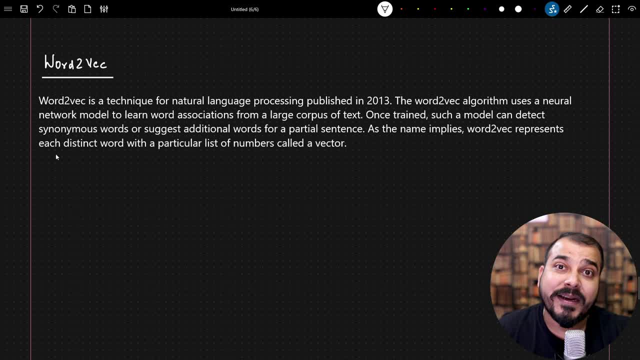 that how word2vec models are basically prepared with respect to architecture in the case of deep learning models, And for that you really need to have knowledge about ANN. you really need to have knowledge about ANN models, right, If you really need to understand that how we can train. 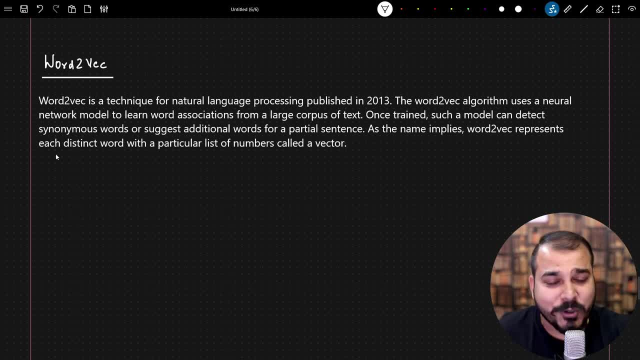 word2vec from scratch. okay, And yeah, let's go ahead and read the definition and let's see that what all problems it actually fixes. So over here, word2vec is a technique for natural language processing published in 2013.. 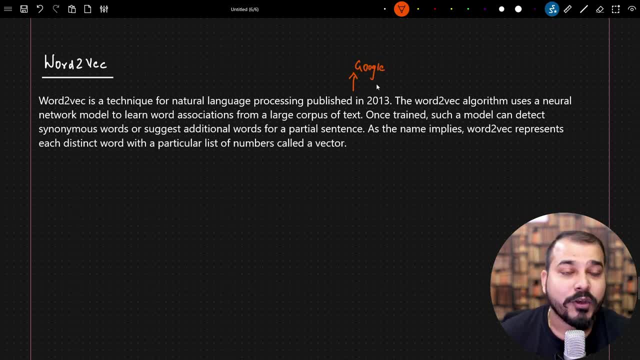 And it was published by Google, an amazing company. already you know that, and they had done some tons of work. with respect to NLP, you know they're doing a lot of research. The word2vec algorithm is based on NLP. 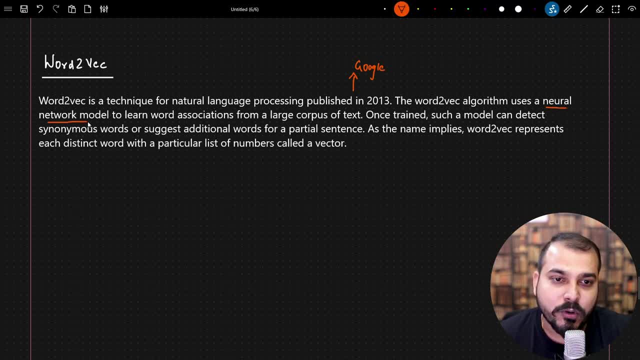 The word2vec algorithm uses a neural network model. We'll be discussing about this, how we'll be using it, how it uses a neural network to learn word association. Please make sure that you understand these words. To learn word association from a large corpus of text. 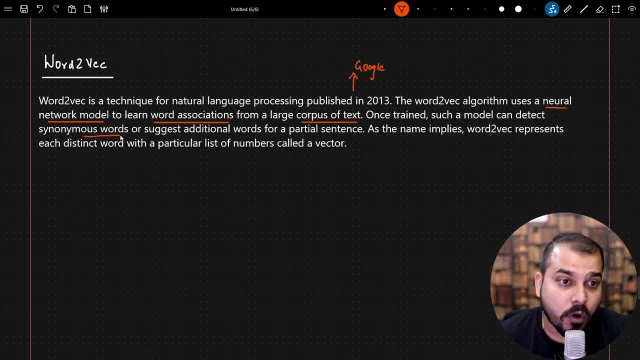 Once trained, such a model can detect synonym words or suggest additional words for partial sentence, So it will be able to detect synonyms. it will be able to detect opposite words and many more things. As the name implies, word2vec represents each distinct word. 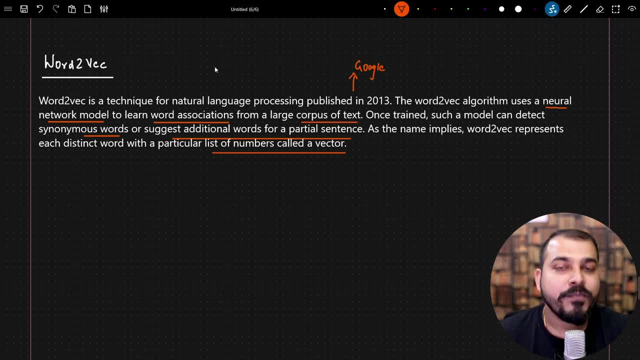 with a particular list of number called as vectors. So at the end of the day, we are converting a word into vectors. but this vector will have many things. It will be able to detect synonym words, or it will also be able to suggest additional words. 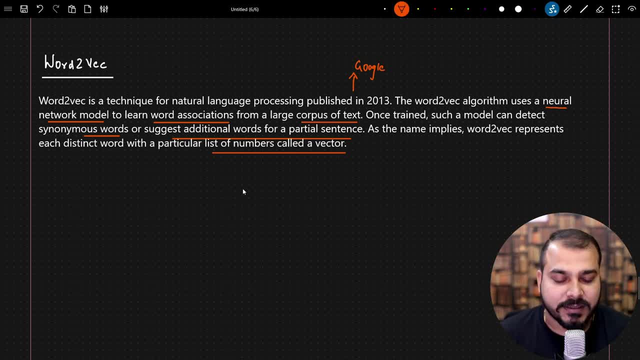 for partial sentence. okay, Now let's understand what exactly this is. Now see guys in bag of words: TFIDF. we have already seen right based on the vocabulary size, we'll either get one Z or we'll get two Zs. 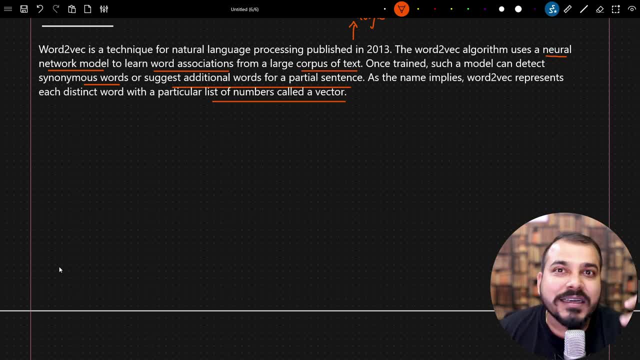 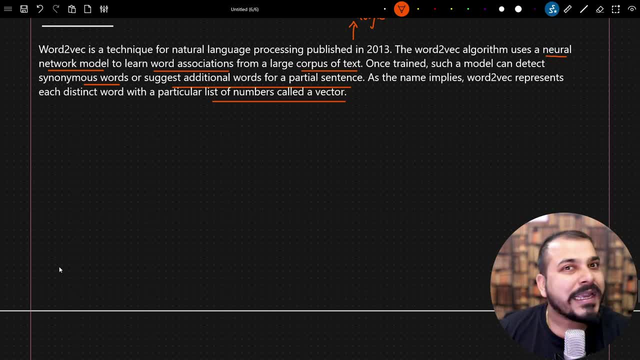 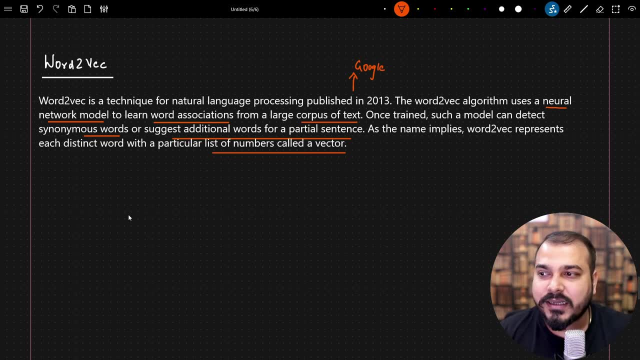 In TFIDF also, we may get decimals like .25, .6.. Then again zeros. zeros are there In word2vec. it'll be a little bit different. Now let me talk about how it'll be different. Let's consider that I have a vocabulary, okay. 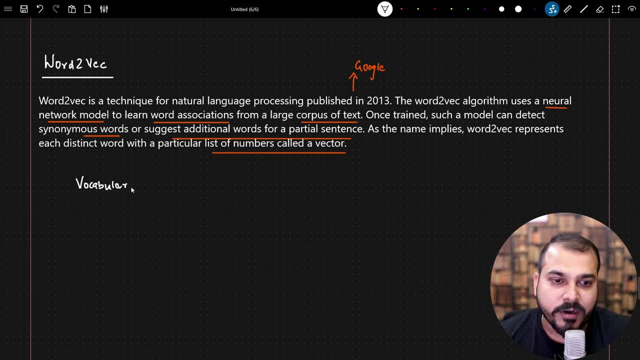 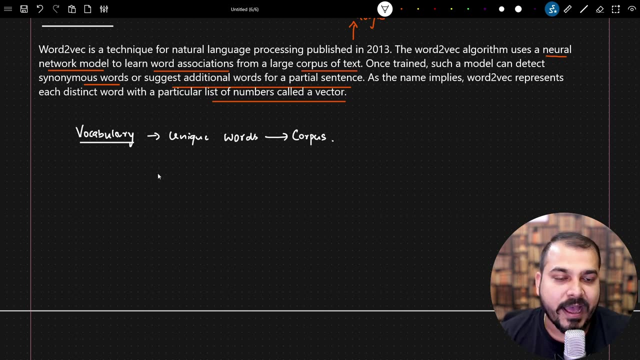 And I have a vocabulary. Let's say I have my vocabulary, So these are basically my, this many number of unique words I have in my corpus. okay, Unique words I have in my corpus. Corpus basically means paragraph. okay, Now let's say the vocabulary words that I specifically have. 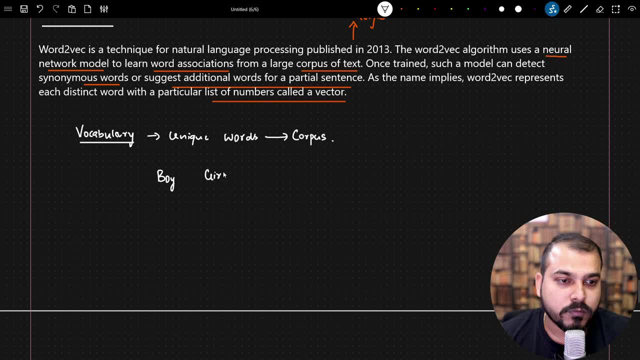 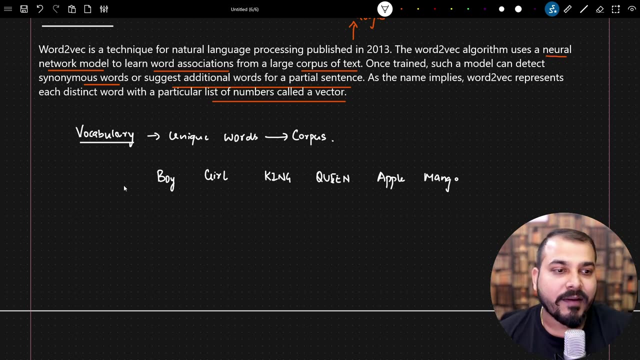 like something like boy, girl, okay. And then we have something like king, queen, And if I probably talk about some more words like apple and mango, Let's say, in my vocabulary I have this many words, okay. Now one very important word I'm going to put up over here. 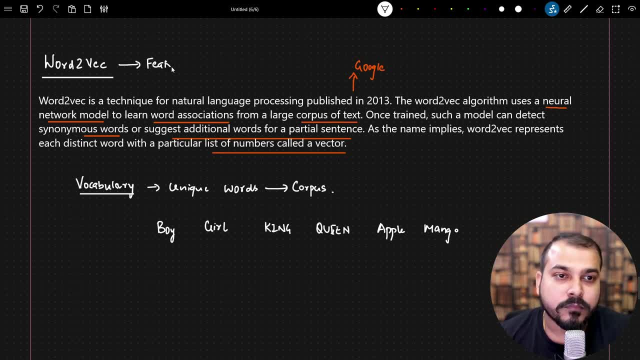 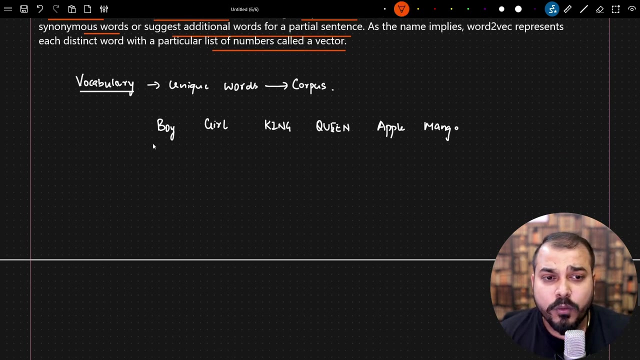 which is called as feature representation. Feature representation- Please listen to me very, very carefully- A very important topic Now. each and every word that are present in the vocabulary will be converted into a feature representation. Now, what this exactly means? This basically means that we are going to convert this. 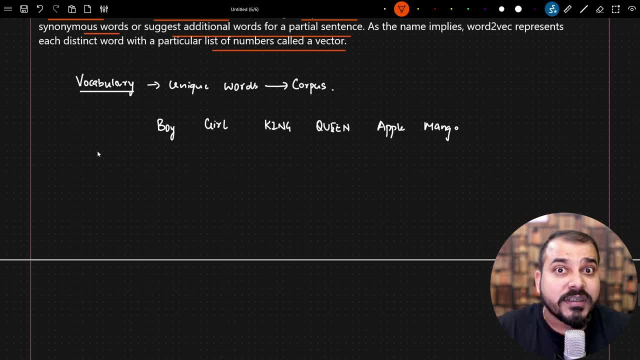 all words into a vectors based on some features. Now, what all features? can it be right? Let me give you a very good example about it, But understand that when we are training a very big Word2Vec model, at that time you'll not be getting a clear idea. 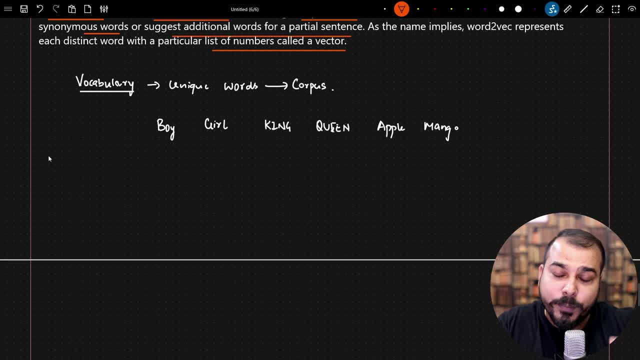 about all the features. But here, just to make this intuition, to make you understand the intuition, let's discuss about this feature representation. So in the left-hand side, what will happen is that let's say that I will be having a lot of features like this: 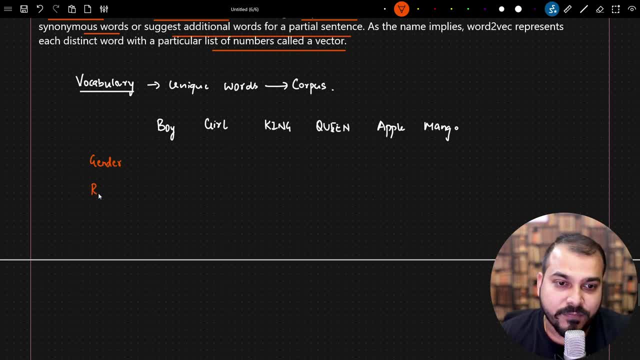 So I may be having a feature called as gender, I may be having a feature called as royal, I may be having a feature called as age, I may be having a feature called as food. Like this, I will be having lot of features. 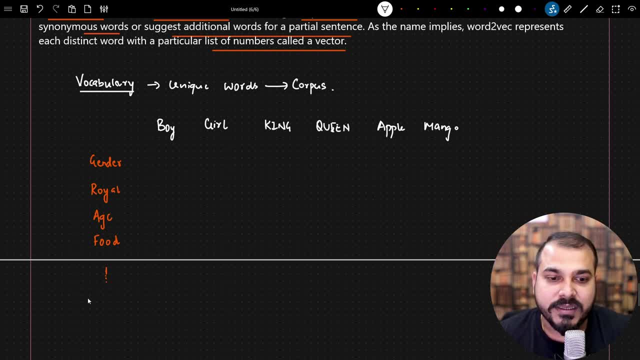 And let's say that the total number of features are basically 300 dimension. That basically means I will be having one more nth feature over here And the size of this entire features, like if I probably count all of this, This will be 300 dimensions. 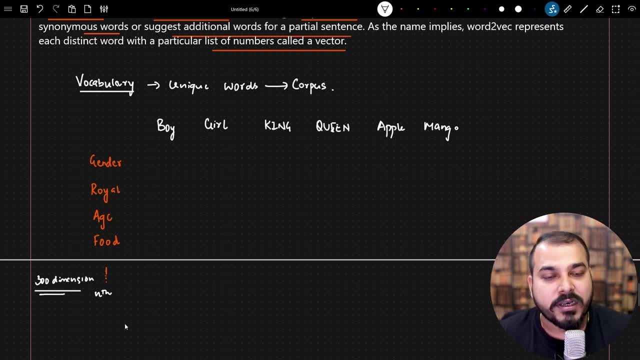 Let's consider 300. Dimension basically means I will be having this 300 features. Now this vocabulary, we are going to represent this word in the form of vector, considering this feature representation. so this is my entire feature. okay, what i'm actually going to do? i'm going to take up 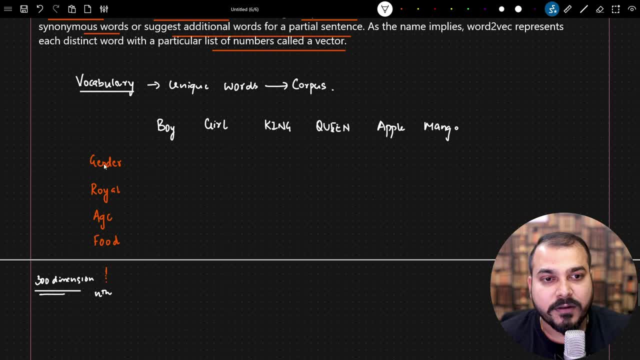 all these words that are present in the vocabulary. based on this particular features, we are going to assign one numerical value. okay, and understand one thing: this numerical value will be assigned based on the relation of these two words, that is, the vocabulary and this feature representation that we have here. i have given you as an example, but when we are training a very large word2vec, 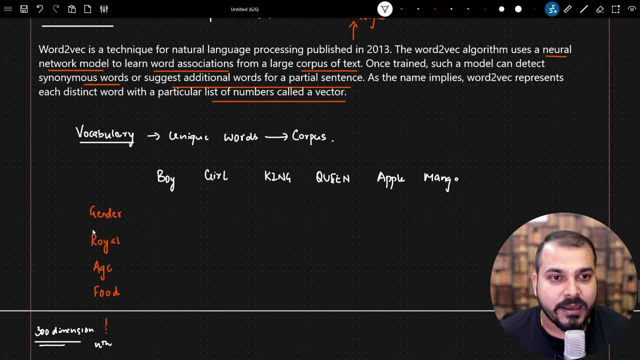 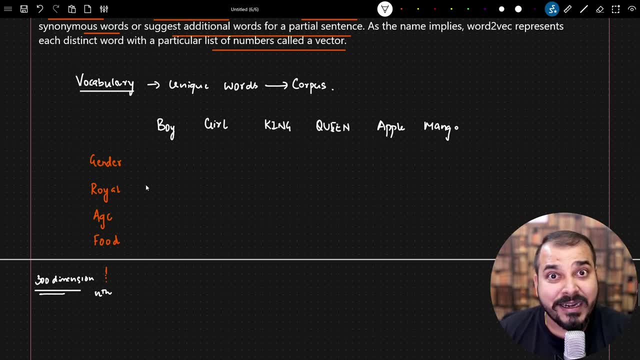 model, we will not be able to see these features entirely, right? if i take an example of google, you know they have come up with this amazing word2vec model which is basically trained in 3 billion words. i guess 3 billion words which is coming from the news feed, right, and that practical example. 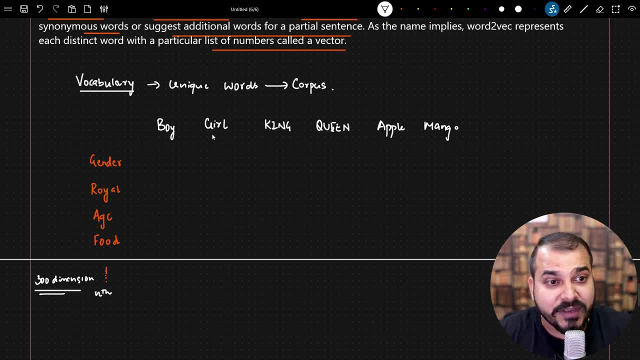 also try to show you- and at the end of the day you'll be able to see- that each and every word is basically represented by 300 words. so you can see that each and every word is represented by 300 words and each word has 300 dimension of feature representation. that basically means every word will be having a 300. 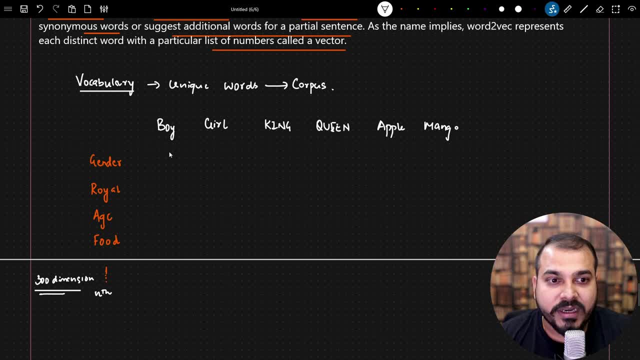 dimension, uh, vectors, okay, now, this is super important. what kind of values that i can have over here? right, what kind of values i can have over here now, let's say, with respect to boy, which is present in the vocabulary, okay, and it's and it's relationship with respect to gender. let's. 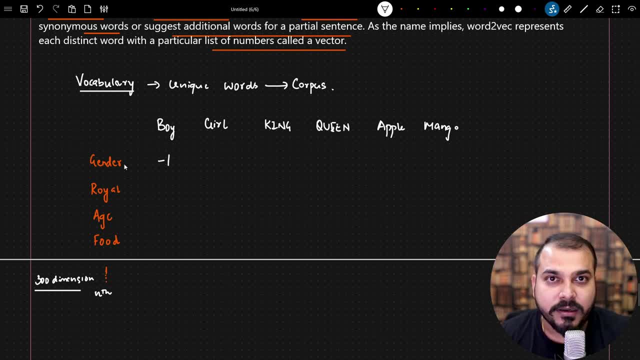 say that i'm having one minus one over here, let's, let's. let's just consider: okay, minus one over here, value can be plus one, because it is the opposite of boy, right opposite with respect to gender. if i say boy, is there opposite of boys, nothing but girl. so minus one and one. this kind of vectors can come. 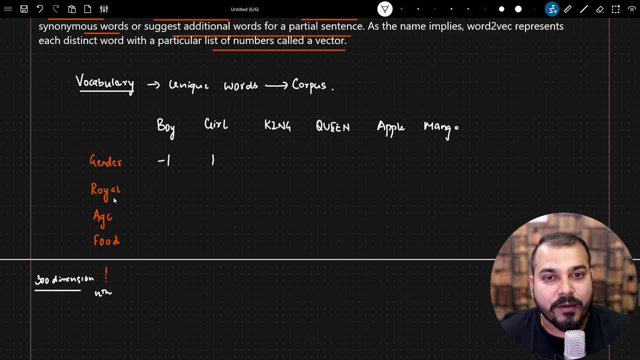 now here you can see, with respect to the next word over here we have boy, we have royal. we obviously know we cannot say, right, we don't have a sentence that, oh, he's a royal boy, he can be a royal prince or he can be a royal king, right? so there is no, no proper relationship. so in this particular case you 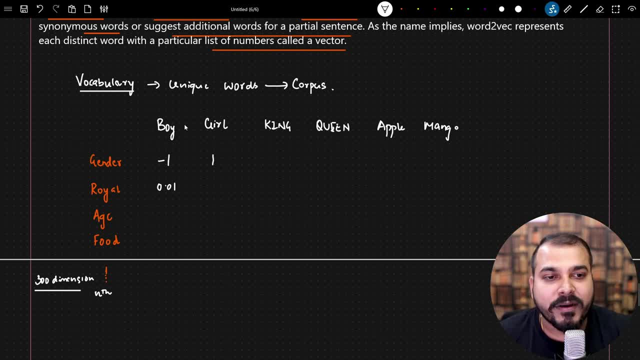 can have that as a point: zero three, okay, so i'm giving you as an example, right. similarly we will also be having with respect to boy and age. let's say that there is not much relation, so i'm just going to put it as 0.03. okay, very near to zero now. similarly, i can have all these values over here. 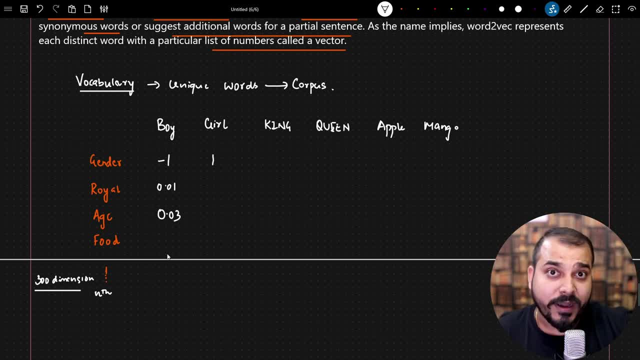 and these all values comes through proper trained models like word to work, word to work which is trained by deep learning techniques, like ann. okay, and i'll show you in the next video how those models are basically trained. but just understand, over here, each and every that we are seeing is represented based on this feature representation. so that basically means 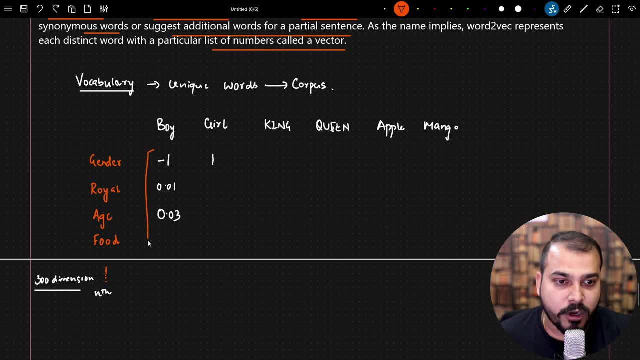 for boy, i will be having this vector. so for boy, for boy, you can see over here, i will be having this specific vector. okay, so this, all vectors will be here, okay, now. similarly, with respect to girl, now you can see with respect to gender, if boy is having minus one, then this will. 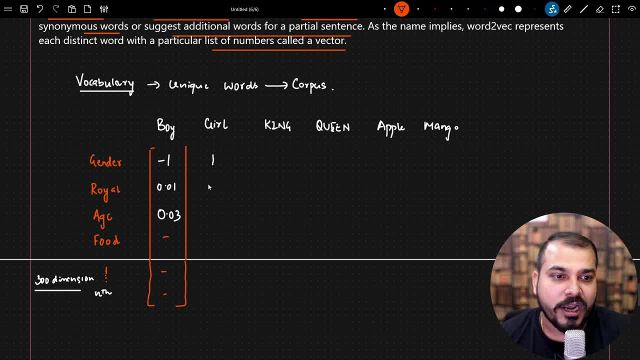 be plus one. right, because it is completely opposite. with respect to royal, again no relationship. so it is yours, so we do not need to find a better way to handle this. because it is also fine, let's say here i'm going to put point zero. two because age: with respect to this, also, no specific relationship. 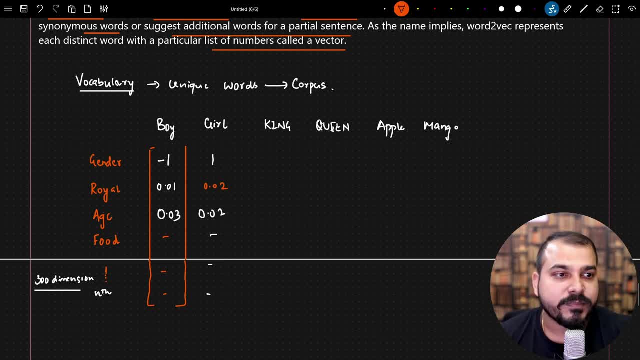 right. so similarly i will be having other values like this. now see, with respect to king, you know i may have gender like: uh, there is a relationship with respect to gender and king, so minus 0.92 will be there. with respect to quin, it can be plus 0.93, you know. so here you can see opposite, right? 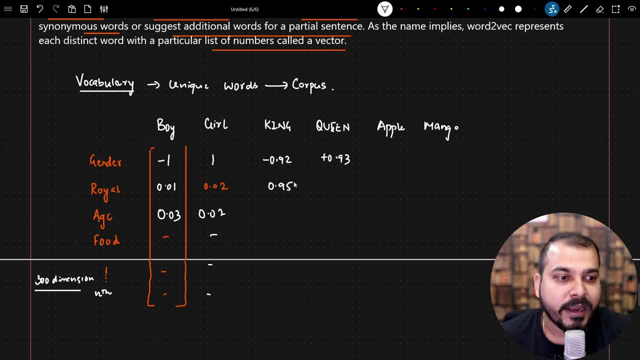 opposite, opposite over here right. and similarly i can have other vectors, like over here royal and king would be more 우ك related right, so i can have 0.95, okay, and over here you can see also royal and queen can also be a royal right. so over here probably the value can be 0.96. 0.97, very much nearby each other, right. 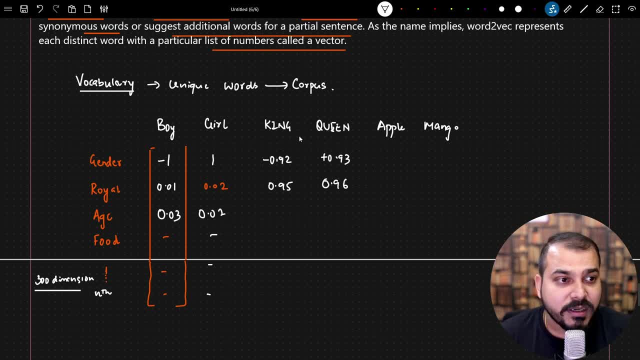 now understand because of these vectors you know, similar words will be, will be very, very close to each other, because if i try to subtract it, i'll just give you an idea about it. so right now, with respect to age also, obviously there will be some relationship between age and king, because we say: 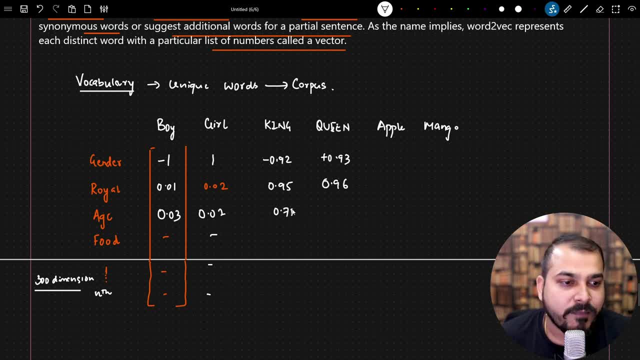 that old king right with respect to age. so suppose let's say: here i'm having 0.75, here i'm having 0.68 and like this i will be having multiple vectors like this right and we can clearly see right over here it is now see with respect to apple, obviously it will have no relationship. 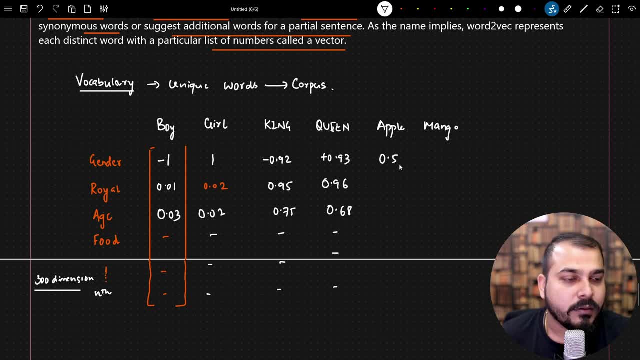 with respect to gender, uh, gender, so i can probably write 0.5 or 0.01, something right. with respect to mango also, it cannot be so i'll write just 0.23. i'm just saying that, okay, we basically, uh, can have some values over here. if it is not having a relation, it will be very. 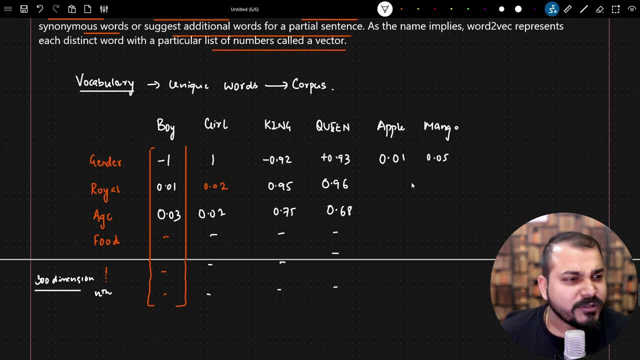 much near to 0, like 0.05. okay, i'm just putting some values, but once we train all these models right, we will be getting this value here. i'm giving you a crux idea about, like, how each and every vectors may look like. okay, now over here with respect to apple and royal. also, i'll not 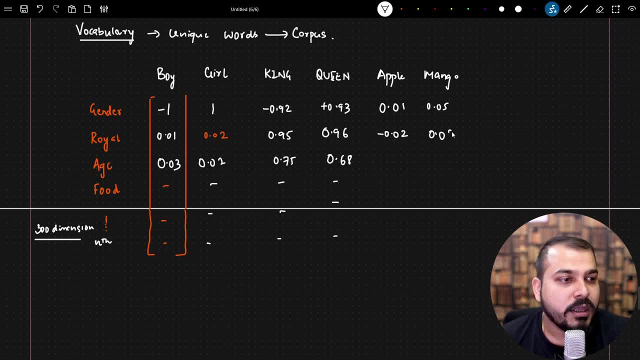 be having much relationship. so let's say i'm putting minus 0.202. this will be point plus 0.02. with respect to age and apple, this may have a very good relationship, right? because uh, let's say, if the apple is kept for 10 days outside, you know, it may. 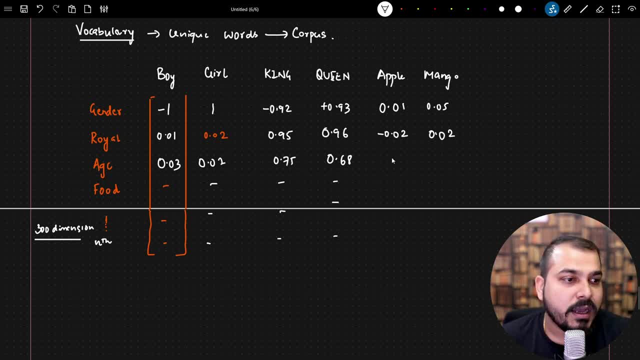 it may rotten up, right, it may not have that nutritional value. so this, uh, with respect to age, it may have a direct relationship. mango also may have a direct relationship, so we are going to have this vectors pretty much similar. with respect to food, yes, apple belongs to a food item, right? so 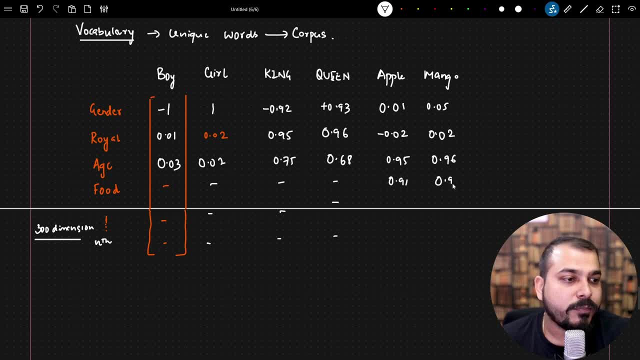 this will probably have a good value. it may be 0.91. this is also 0.92, right, and similarly i'll be having different, different vectors, right. so here, what we have done is that each and every vocabulary word is represented based on this feature: representation. 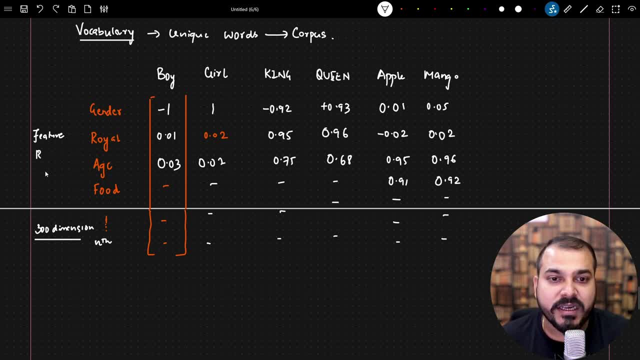 right, and here the feature representation may not only be 300 dimensions, it can be 100 dimension, it can be different, different dimensions, right, but here i'm just saying, showing an example, with respect to google and what will be these features. that will also not be exactly, no, but just consider. 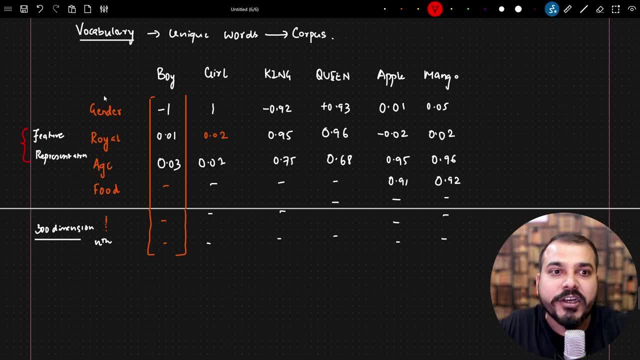 that- i'm just giving an intuitive example- that, yes, based on some relationship with respect to the word, you are able to get this: specific vectors. now, there are a lot of advantages with respect to this. you know why i'm saying you? because, suppose, let's say, if i do a calculation which is like king minus man plus queen. 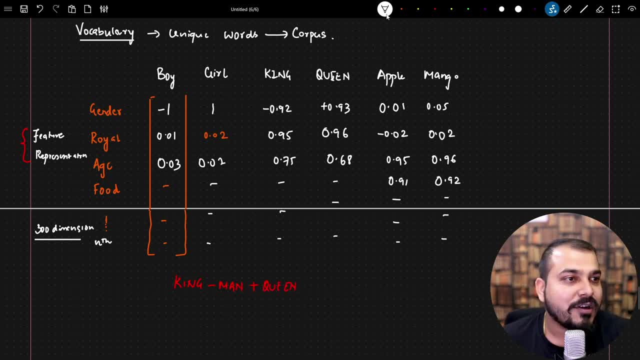 if i do this calculation- and this is a famous calculation which is also written in google research paper- if i probably do this calculation, the output that i'm going to get is something called as woman. okay, i will definitely get it as human. why, all away? human is not there. it's okay. 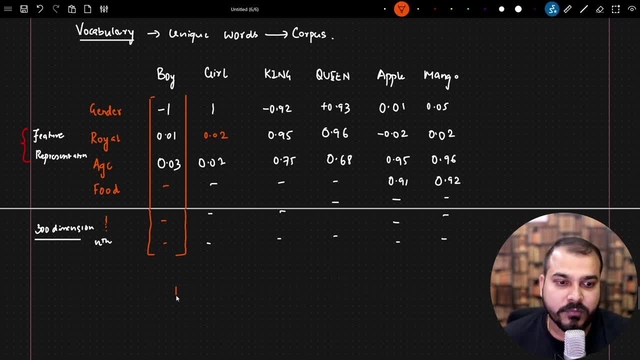 so i'll let me just remove it. suppose if i say king minus boy plus queen, then the output that i'm going to get, see king, is this vector right? i'm subtracting with boy and then i'm adding it up queen. at the end of the day, you'll be seeing that. 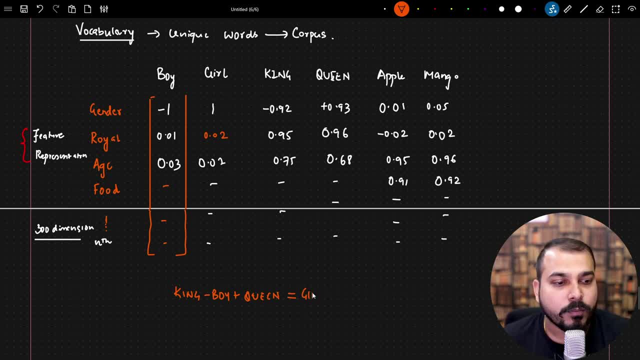 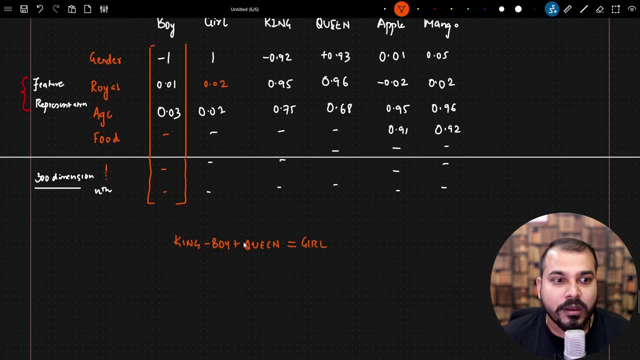 the girl will be much more related to boy, so i'm going to get the output as girl here. i'm just doing the vector calculation and this is what kind of relations we'll be able to get. it, you know, this is what this is is an amazing thing. we are getting this kind of relation just by seeing these vectors, which has 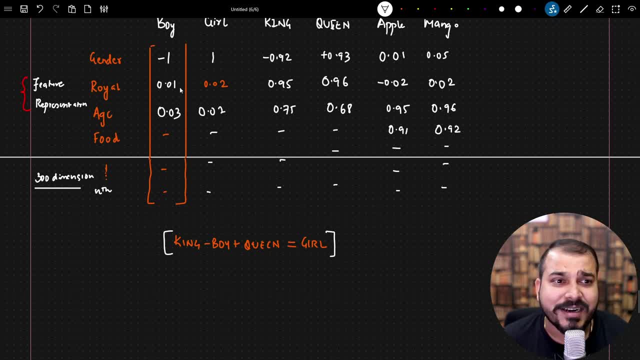 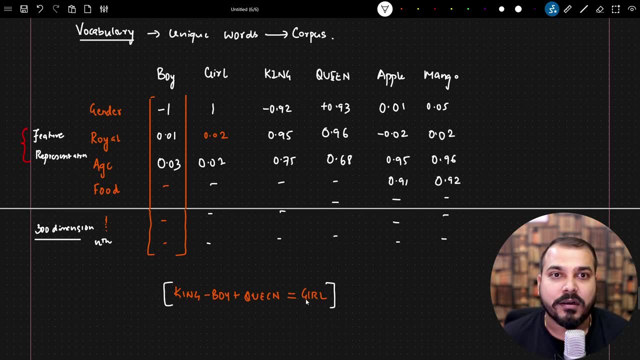 been provided by word2vec. again, i'm not going to do the calculation here, i've just randomly stuffed some values. but in the real word2vec use case you'll be seeing that if you do this kind of calculation you're going to get good. and this i will show you practically also as we go ahead. 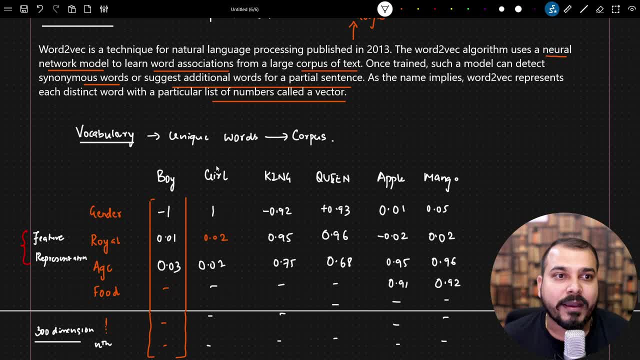 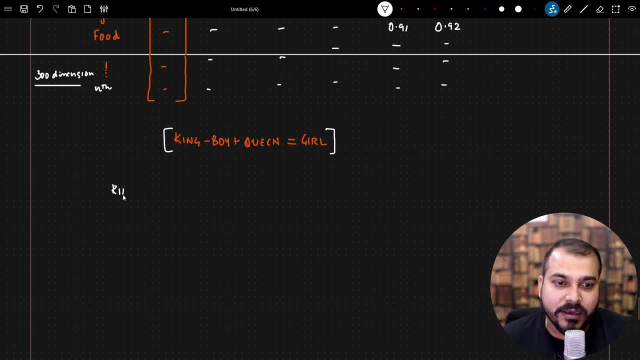 once we use this google, uh, google word2vec, which is basically trained on three billion words, which is quite amazing, right? so let me give you another example. let's say here what i'm doing. instead of using 300 dimension, i'll represent every word by two. 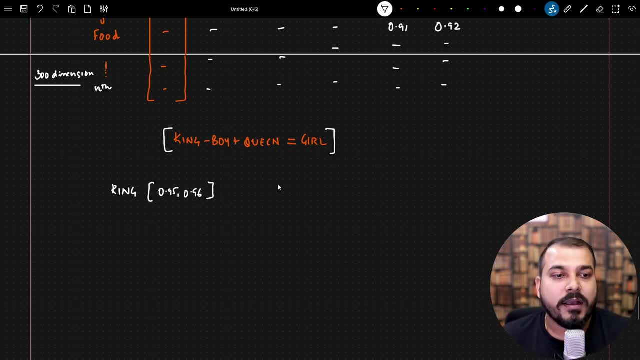 dimension. let's say i have 0.95, 0.96. man is represented by something like 0.95, 0.98, let's, let's represent like this: okay, i'm just giving some values, okay, some meaningful values, so that you'll get an idea about it. let's say, queen is given as 0.96. let's say, because this is the 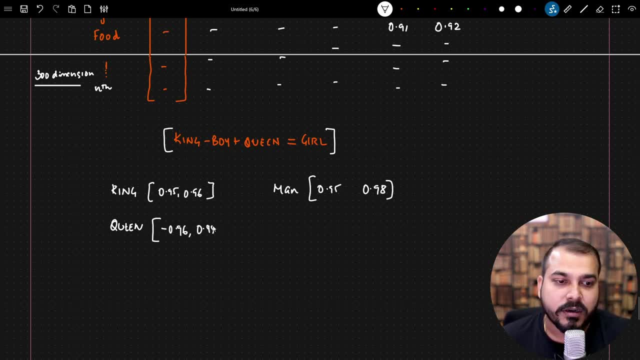 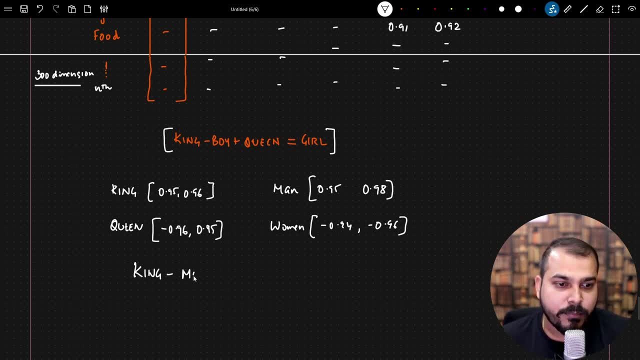 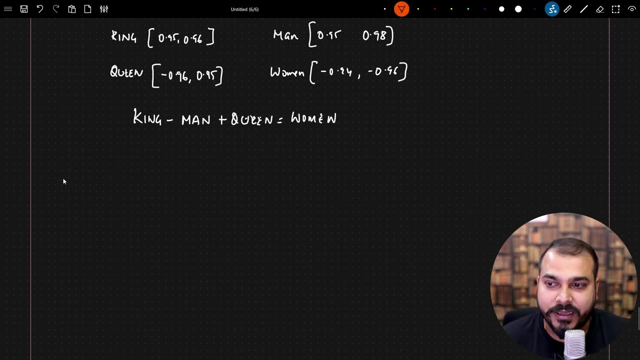 we do the calculation of king minus man plus queen, i'm going to get the human right as the output. now, what this vectors represent, that also you really need to understand. it is super, super important, and that is where i'm going to discuss about something called as cosine similarity. 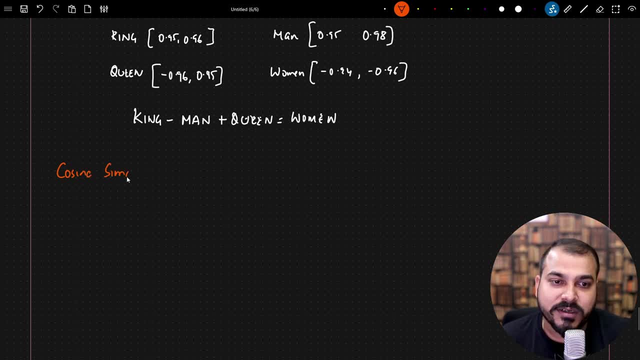 okay, cosine similarity super important. okay, cosine similarity super important with respect to understanding these things. because if you understand these things and all now see over here, king is given by two, two, two vectors right: 0.95, 0.96. so obviously i can, i can. 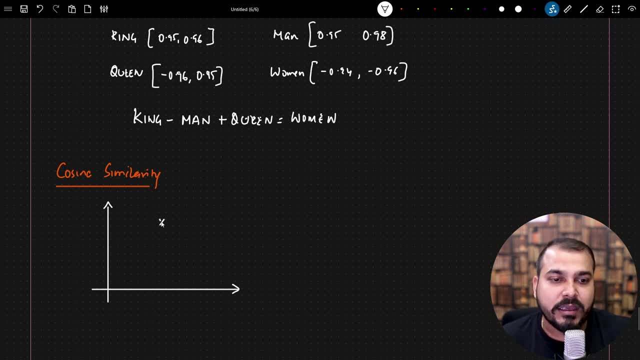 basically construct this into a two dimension. let's say that i'm getting king over here, okay. and in order to make you understand, let's say queen is over here, okay, or queen can come over anyway. let's say man is over here, right, man is over here. if i probably say king with respect to 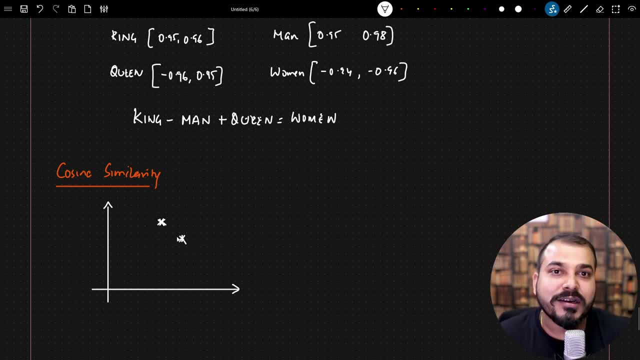 gender right, this two is going to be the most nearest word when compared to queen right. so if, how do i calculate the distance between this vector and this vector, which is provided in this form? all i do is that i try to probably calculate the distance like this. okay, i try to find out. 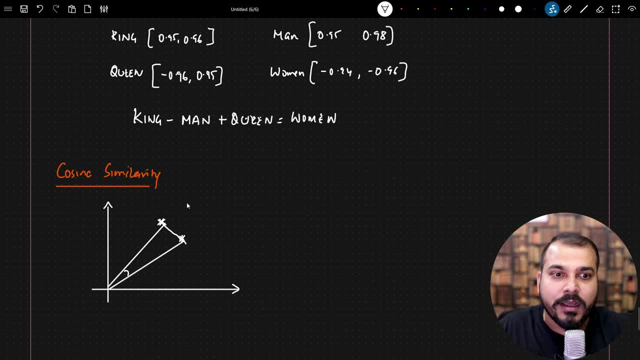 the angle. and for this, to find out the distance between two vectors, we use a distance formula which says it is nothing but one minus cosine similarity. now, what is cosine similarity? this is super important to understand cosine similarity. i can basically say that cosine similarity is nothing but cosine similarity is nothing but the angle between these two vectors, let's say the 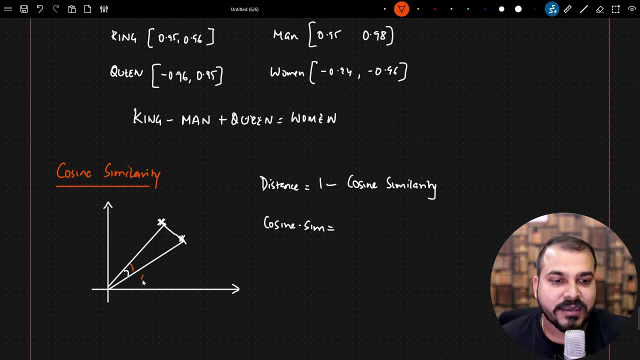 angle between these two vectors. let's say- i'm just taking as an example- is 45 degree. let's let's consider then: this is nothing but cos 45. cos 45 is nothing but 1 by root 2 and probably, i think this is approximately equal to 0.7071. i've done the calculation. if it is wrong, just let me know, okay. 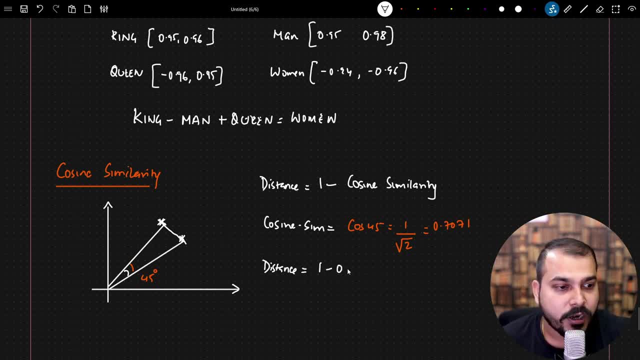 the distance between these two vectors will be nothing but 1 minus 0.7071.. Now, if I'm calculating the distance, it is 0.29. let's say So. if I'm getting this 0.29 distance right, I will say: 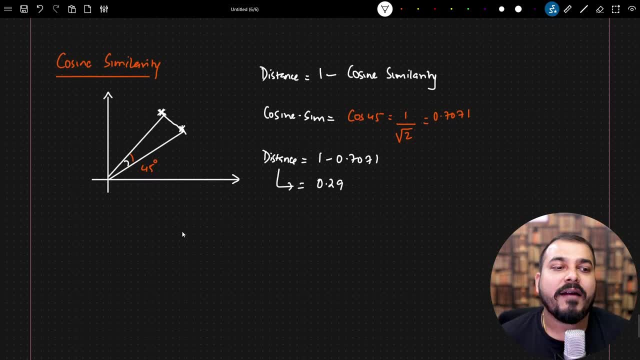 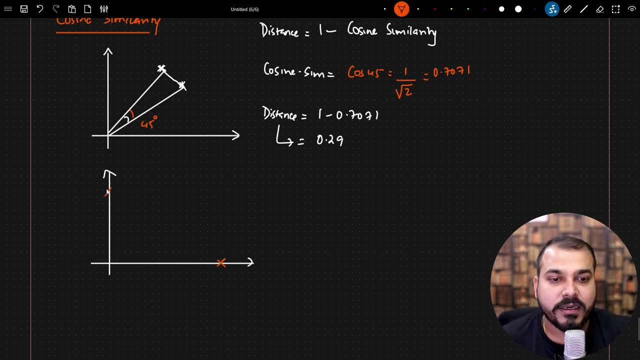 that- okay, almost this particular word- are similar. Let's say, if I have two more vectors, if I have two different vectors, one of the vector is basically over here, one of the vector is over here- then the angle between these two is nothing but 90 degree. In the case of 19 degree, my 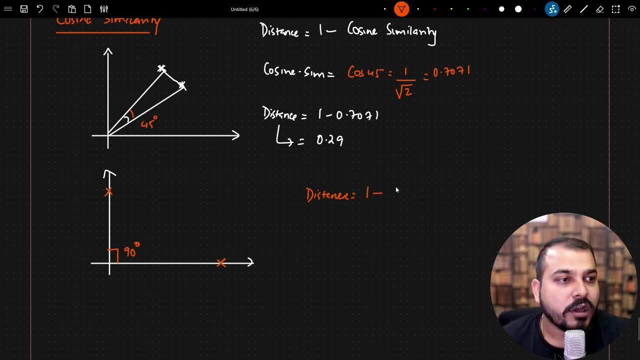 distance will be nothing but 1 minus cos theta. Cos theta is nothing but cos 90.. Cos 90 is nothing but 0.. 1 minus 0 is 1.. So I can definitely say this vector and this vector are completely different. 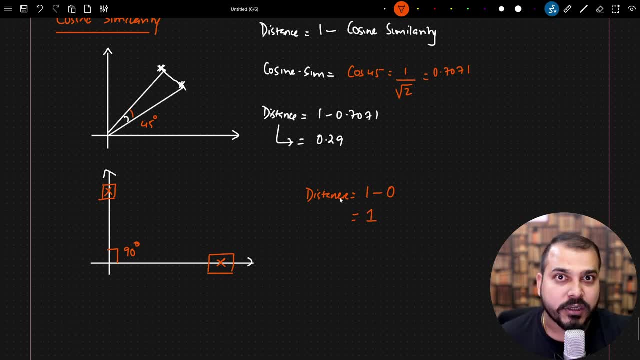 because the distance between them is 1.. If the distance is nearer to 0, I will say that they are almost similar vectors. Now, in this case it is 0.29.. I can say that, okay, somewhat similar, right? Let's say, if I have one more vector which is in this point, only then I can say that these 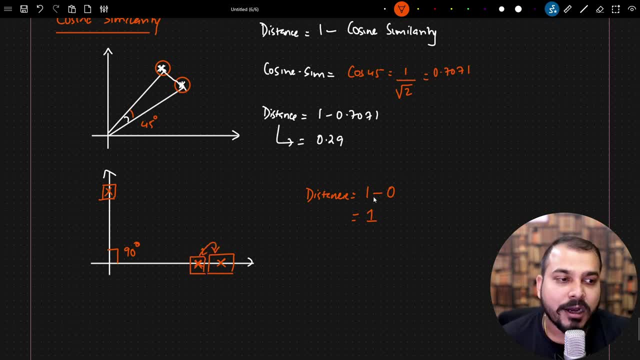 two vectors are almost same because the angle between them is 0.29.. Cos 0, cos 0 is nothing but 1 minus 1, which is nothing but 0, right? Because over here the angle between these two point is nothing but 0, right, There is no angle at all, right? So if 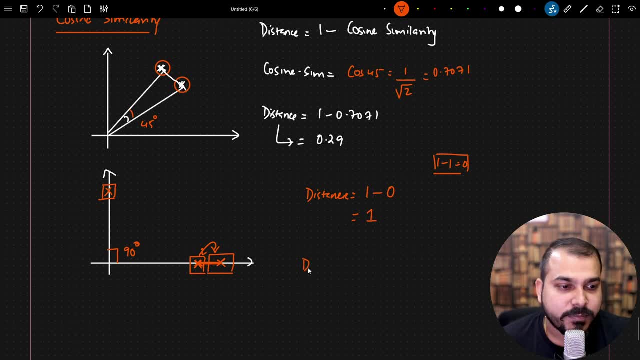 there is no angle, then I will be able to find out the distance. In this case, my distance will be nothing but 1 minus cos 0.. 1 minus cos 0 is nothing but 1 minus 1, which is nothing but 0.. 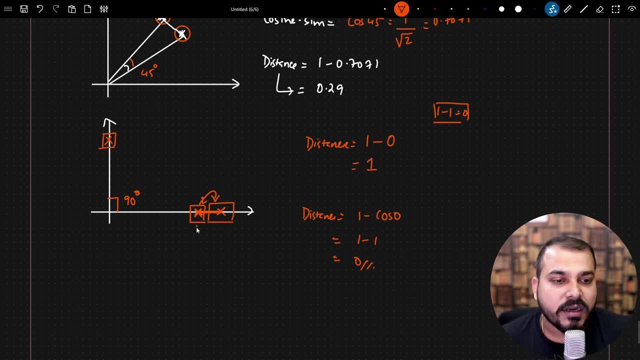 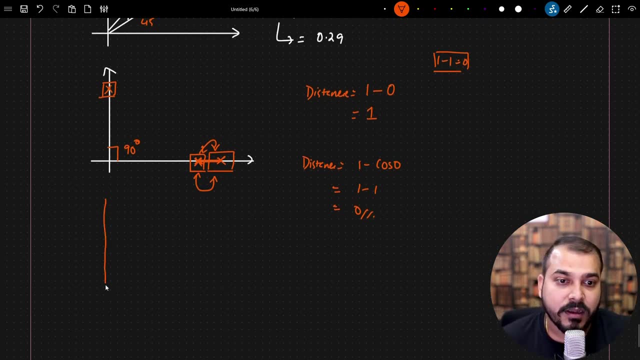 Now, if the distance is coming as 0, that basically means these two are same word. right Now, this super important, because recommendation also happens in this way itself. Now, in recommendation, let's say I have a movie which is like I have Avengers. Let's say: Avengers is over here. Where do you? 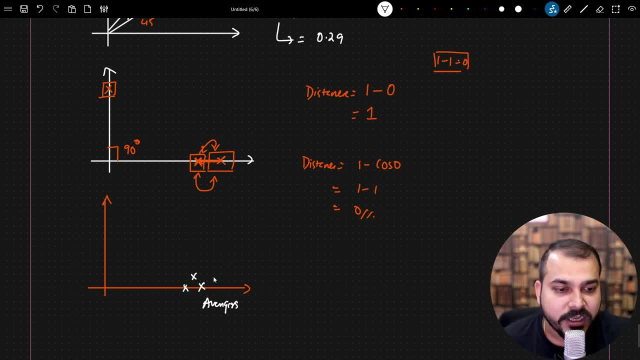 think Iron Man will come. Iron man will come again, near this or near this, at this particular point only, right, Iron man will be coming and it will be based on different, different feature representation, right? Whether it is a comic movie, whether it is an action movie. So action comic. 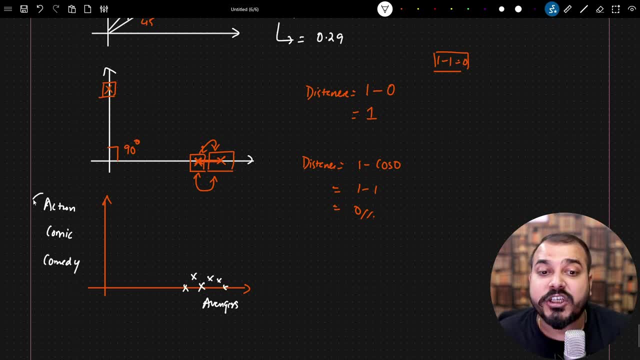 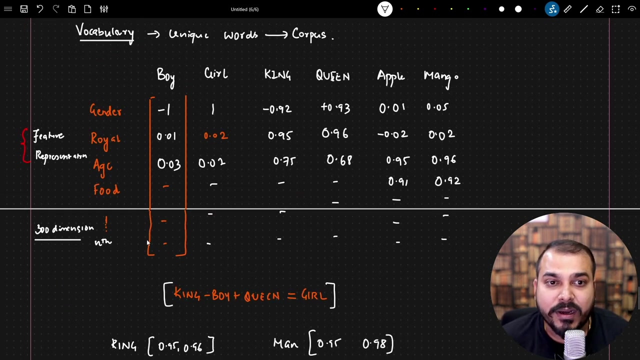 right or comedy. These all are feature representation. Try to understand this. And movie name is basically my vector, my vocabulary. It can be Avengers, It can be this one, right? So I hope you're getting an idea about how word2vec is basically working. At the end of the day, we are basically creating 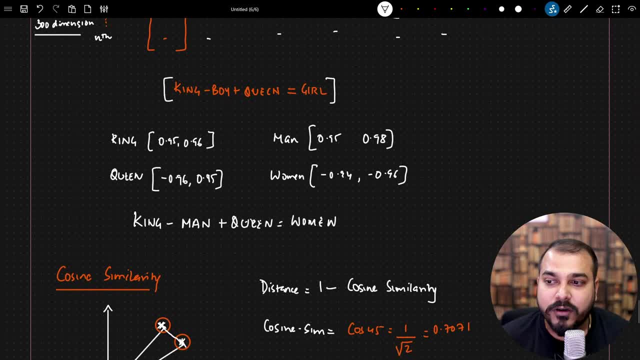 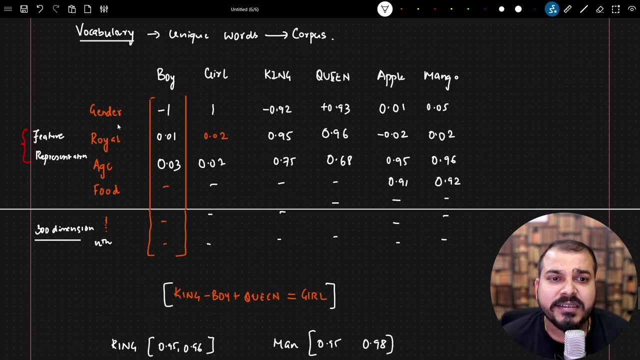 a feature representation of every word. okay, And we are able to find it out. So, yes, this was about word2vec. Now what we are going to do is that you need to understand that, how this feature representation is created and how this vectors is basically created, How this vectors, Because 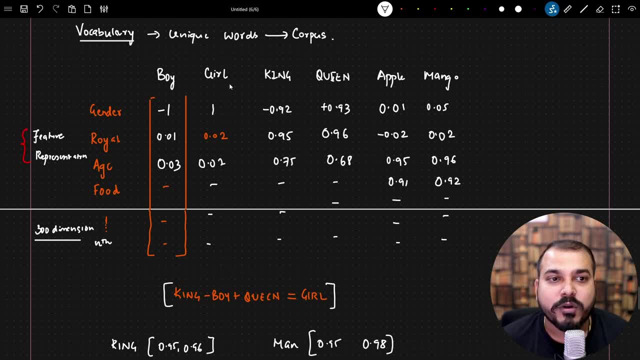 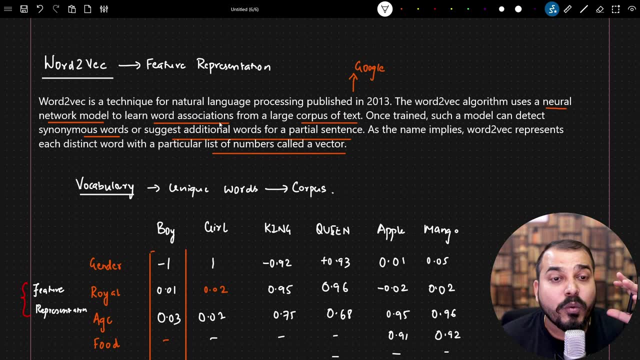 here I have randomly written: boy to gender is minus one, boy to girl, girl to gender is plus one, because I said that, okay, this may be the opposite one. Now you'll get an idea that how, in a deep learning neural network, basically a simple neural network, how this entire word2vec is trained. 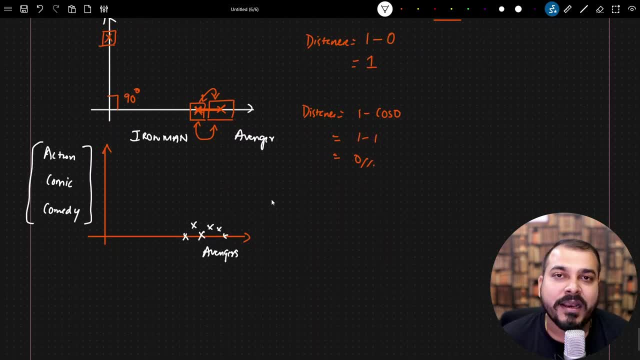 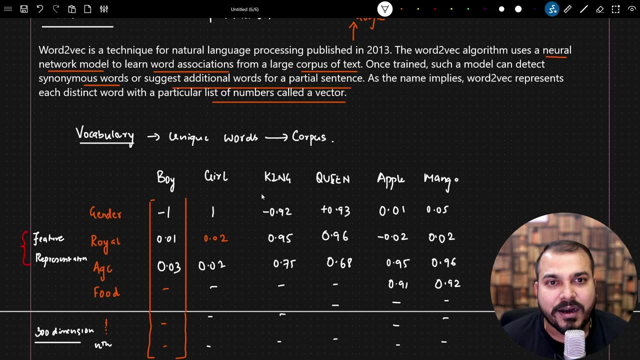 And that is what I'm going to discuss in my next video. Then I'm going to also show you the practical implementation. So I hope you're able to understand this. with respect to this, a very good, amazing model developed by Google, a very good architecture for with respect to this- And we'll 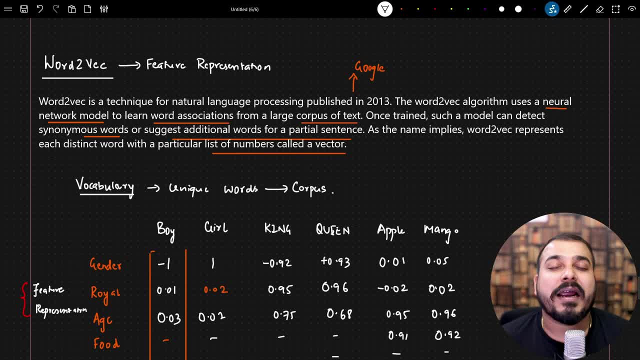 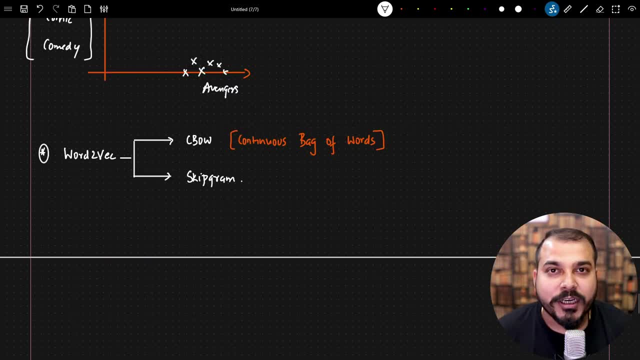 try to solve that in the upcoming video And I'll I'll give you a clear idea about it. Okay, Just the prerequisite is that you really need to know about ANN loss function optimizers and all. Hello guys, So we are going to continue the discussion with respect to word2vec. 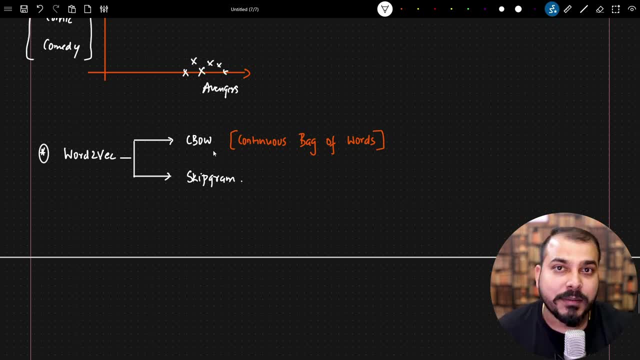 Already. we know word2vec are basically of two types. One is CBOW, which we have already seen previously: continuous bag of words and skip gram. In this video, what we are going to do is that we are going to understand that how word2vec model is basically created. What is the deep learning? 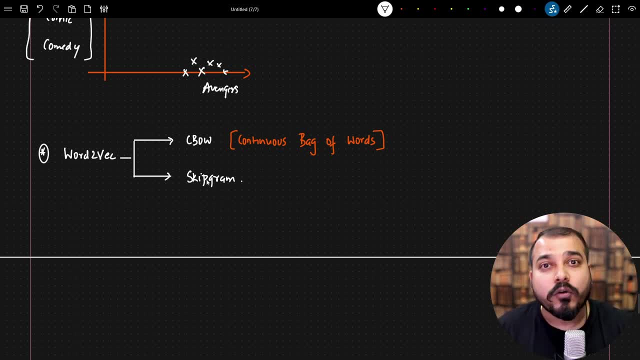 model that we are specifically saying. you know how the inputs and outputs are there and how the model is basically trained. One important thing is that you really need to have a prerequisite knowledge about ANN loss function and optimizer. So let's get started, Let's get started. So let's. 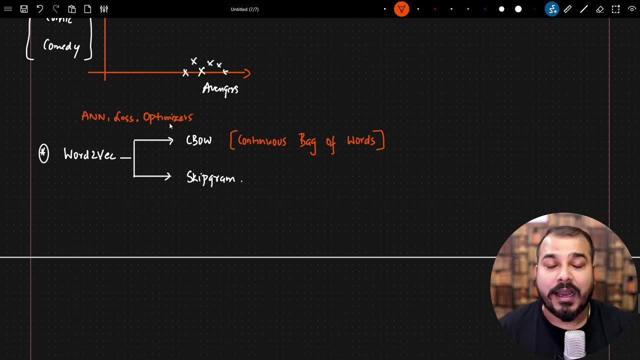 get started with the Flight. I would suggest, first of all, please make sure that you have some knowledge about this right Before you understand this now. with respect to word2vec, one more important thing is that in what to where we also have a pre-trained models right. 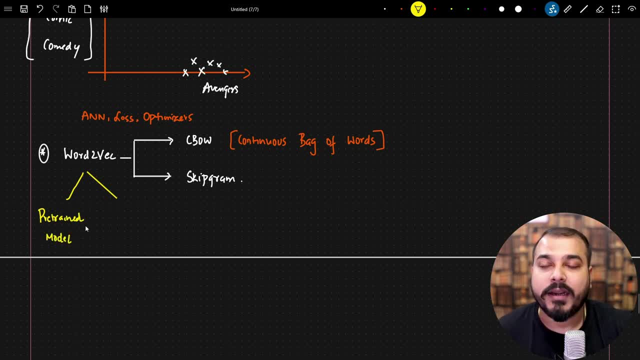 Now, if I talk about a pre-trained model like Google, right, Google has a pre-trained model with respect to what to work, which is straightened on three B, three billion words, And we can also train a model from scratch辛. a model from scratch, right? I have no idea what's. So first of all, just to give you an idea of where we are as a real volume: A few hours ago there was a one click here, a live writing class in the region, or even one in the. 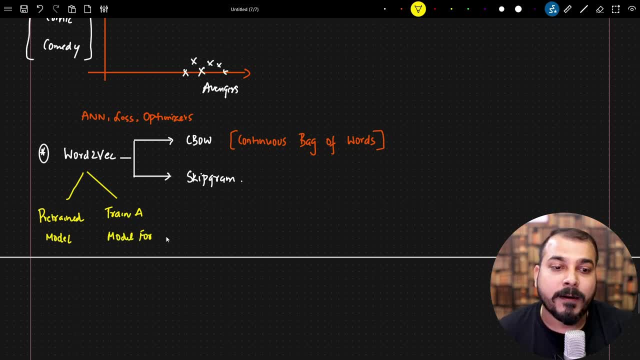 region, in the region Right Now. if we look at the data here, this is what we were looking for. We scratch. okay, and again the reason why I am taking this, because you really need to understand that how that feature representation is basically getting. 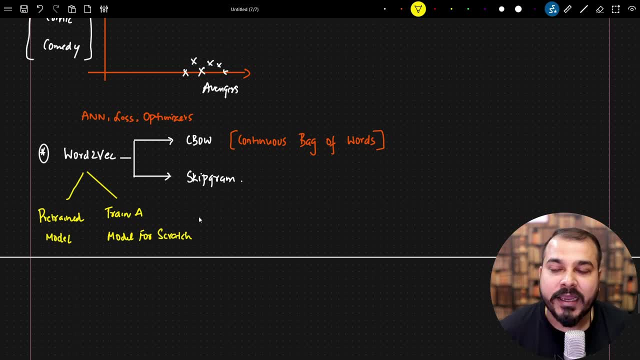 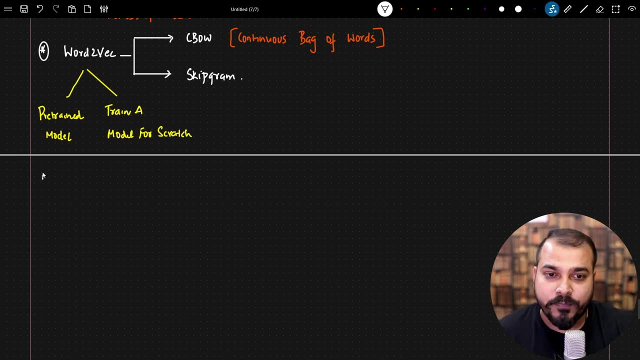 created. okay, now let me go ahead and let me say is that let me take a simple corpus and let's say that first of all, we'll start with C bow. okay, so we are going to discuss about C bow, which is nothing but continuous bag of words, and 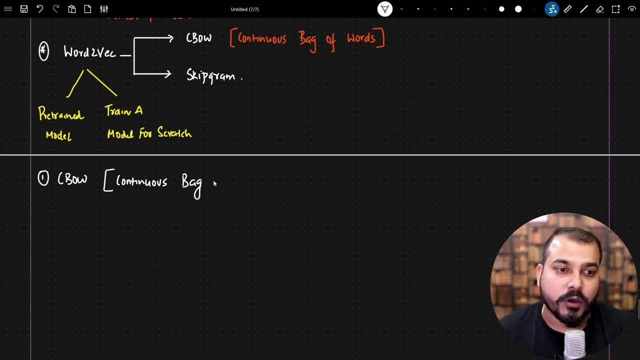 how this model is basically created. it is a type of what do I create? continuous bag of words. now, to solve any problem, I will definitely have a data set. so let's say that this is my corpus, and remember corpus, because all these models, you know, like word2vec is trained on a huge data set. huge data set like this particular. 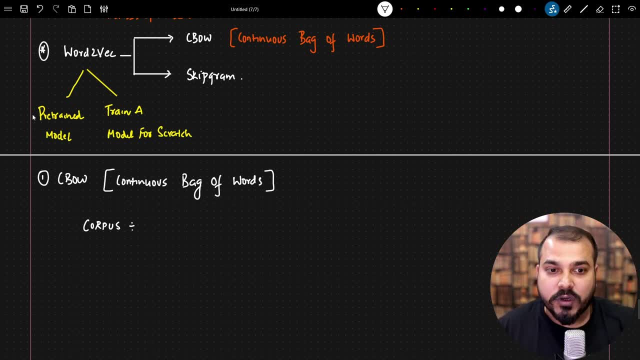 pre-trained model from Google is basically trained on 3 billion words. so let's say I have a corpus or a statement or a data set or or a paragraph. it can be anything, and for just making you understand I'm just going to take a simple paragraph. 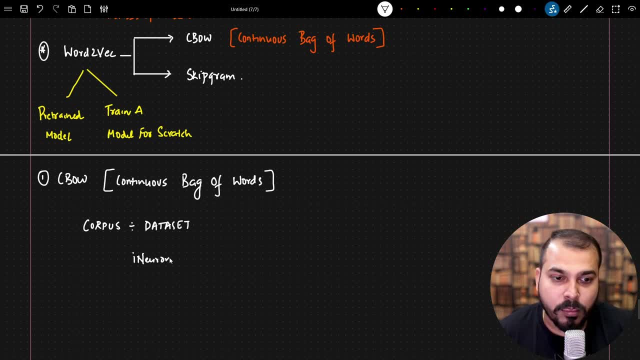 I'm going to say that, okay, I neuron, I neuron is. is I neuron company or I neuron company is related to data science. let's say I have this particular corpus. now remember, like this, in a use case, you'll be having a bigger corpus. it can have millions of words, right? 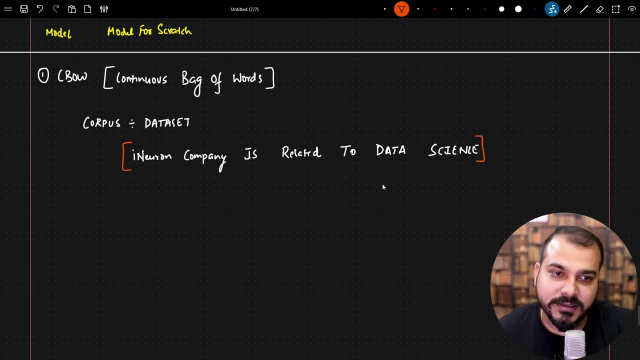 but let's say that I am taking just a simple corpus over here, just a single liner. now we are going to understand that how a see bow word2vec is basically created and how a model is basically trained with the help of deep learning. now, first thing is that whenever we have a corpus, we really need to know what is. 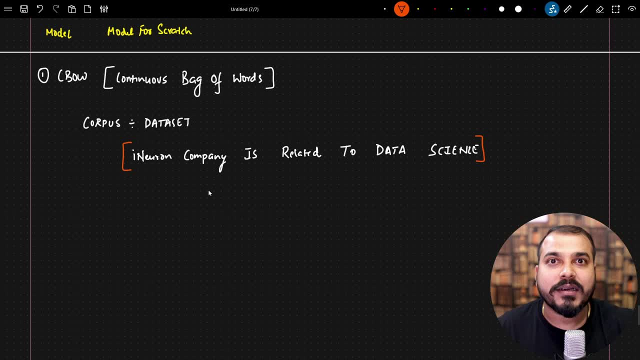 our input data and what is our output data, because word2vec all together is a supervised machine learning, right? so, first of all, what we do is that we select a window size, and I'll talk about this window size and why do I need to select a window size, and I will talk about this window size and why do I need to. 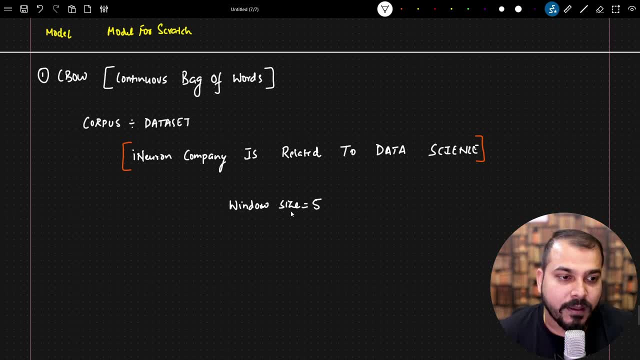 is super important. let's say that i'm going to select a window size of five. now, this window size is super important to basically create your input data and output data. okay, super, super important, like what should be your input data and what should be your output data so that you can train. 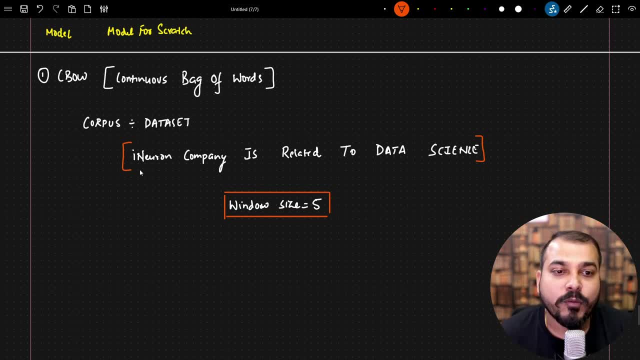 your model right now. this window size five indicates that how many words i need to select initially. so let's say i am selecting five words. so here is my five words now. from this particular five words, i will take the center word. center word. now understand how i will take up this window. 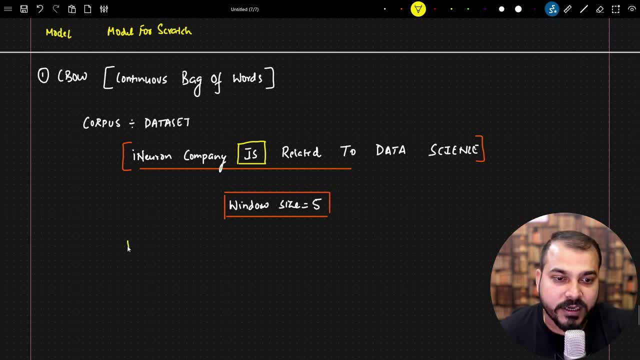 size five words and convert into input and output data. so let's say this is my input data and this is my output data. okay, now the central element that i have actually taken over here is is right now in the input. i will be having i neuron company. 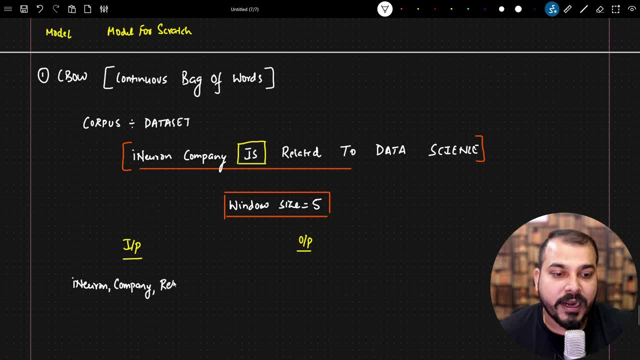 and then, on the right hand side, i have related and i have two. okay, now, why you? why you may be thinking that i'm taking the forward and the backward, because, understand, if i'm taking this as a central word and this will basically be my output word, okay is, okay, this is is basically my output word. now it should be. 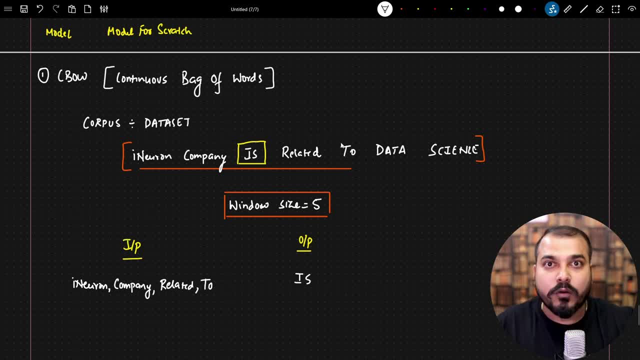 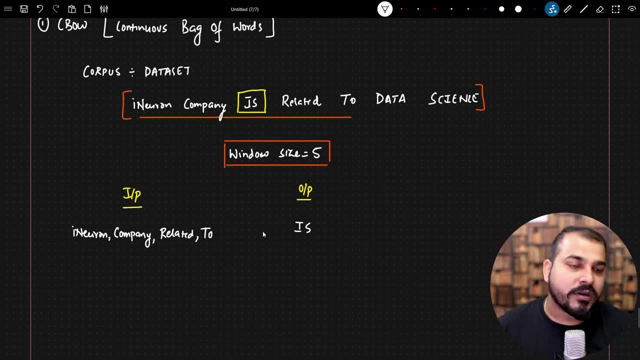 knowing that what all words are in the forward context and what all words are in the backward context. so that is the reason we are creating in this particular way, so that this is output should be knowing about its forward word and this backward word, just to get some idea about. 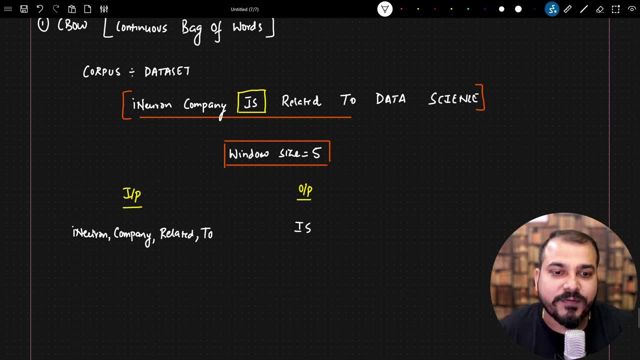 the context of that specific sentence. now, this is the first step. now, when i took the window size as five, the initial five words, i divide my data set into input and output- perfect. now the next step is that i will go ahead and i'll move this window by one step and take the next five words, so the 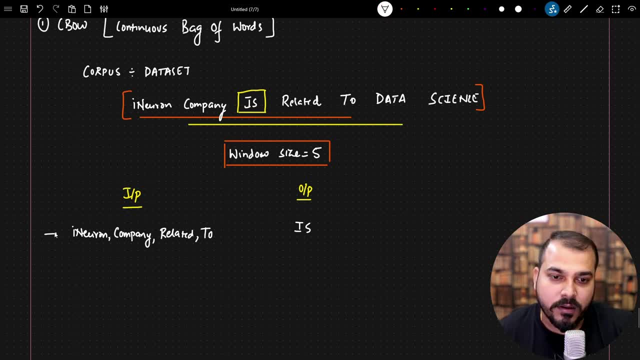 next five words. over here is nothing, but so here this is my sentence one, so sorry, input one, and now this will become my input two, and here i will be having combined company, okay, uh, and again from all these five words, which is my center word. so this is basically. 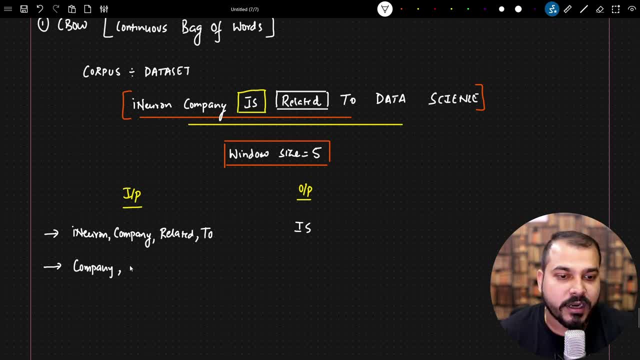 my center. word related, right, so related. so here i'll write: company is uh two and data. so this is my second input, and over here the output will basically be related, right, then, similarly, i will go to the next step and i will push this windows to one step more. okay, so here now i'll be having 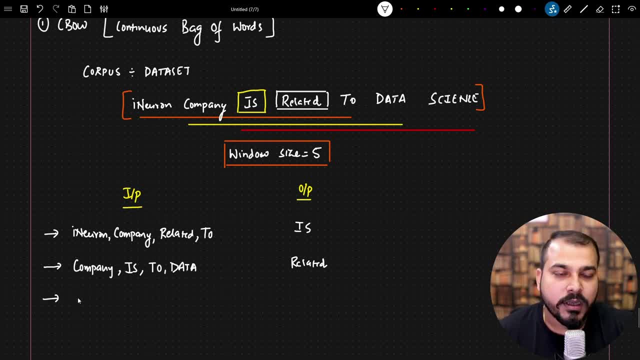 my third sentence with respect to my input and output, and the third sentence again, which is the central word. so this will basically be my central word. so here you have two, okay, and here i'm going to have is related, okay, and then the right hand side data and signs. now you may be thinking krish, should we only take? 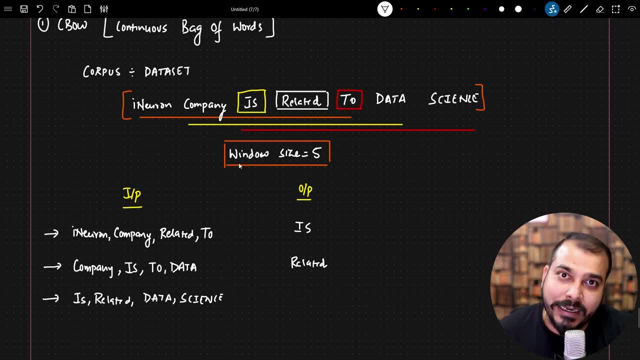 the window size as five. no, you can take any value. you can take any value and why this window size is playing an important role. i'll just say in some time: you can take up any value, but don't take an even number. take an odd number so that i will be getting the central. 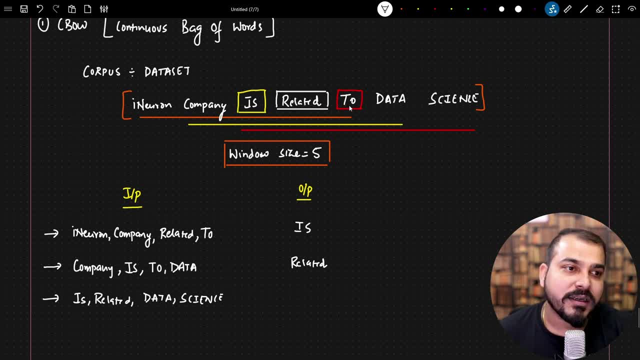 element which i'm taking as an output will have the correct number of words in the forward context and in the backward context. okay, so is related data science is there right now, which is the central word over here? two, right, so i'm just going to write it as two now. this became my input and 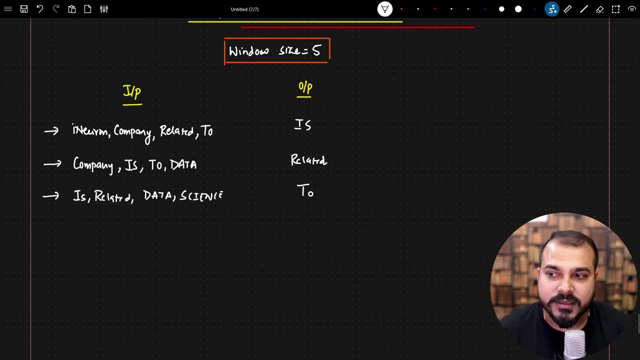 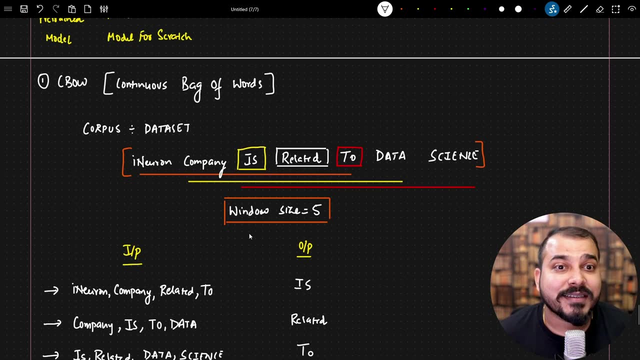 output. now, what i'm actually going to do is that i'm going to train my model with this very simple right. i'm going to train my model with this now: how the training will basically happen and why we do. we say this as continuous bag of words, right, so that part also will try to understand. okay, uh, we'll. 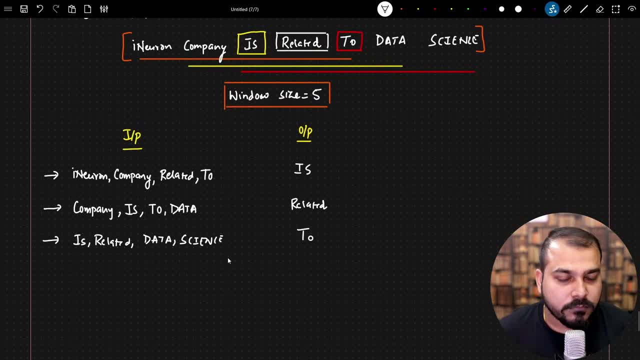 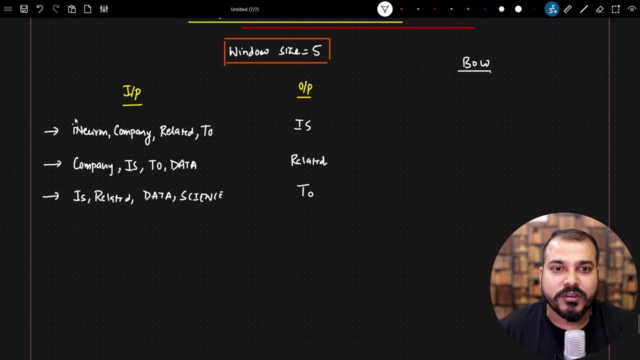 try to understand in a better way now. let's say that, uh, since we are discussing about continuous bag of words, let's say, with respect to bag of words, suppose, if i have this particular sentence right, so let's, let's. let's conclude that i have this many number of vocabulary only. 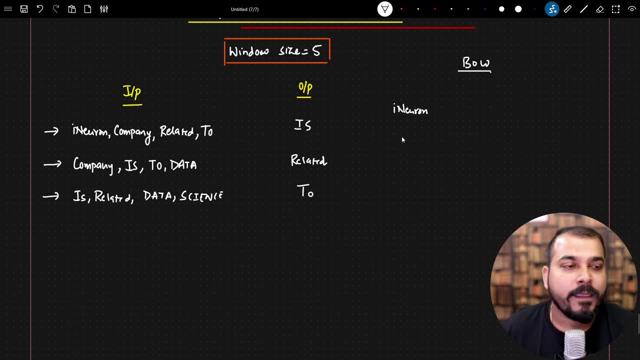 so how many words i have over here, i'm having i neuron, okay, and uh, probably i have company, okay, and i have related and i have two word. okay, now understand this. okay, this is super important to understand. you need to understand that. how many vocabulary of words are there? 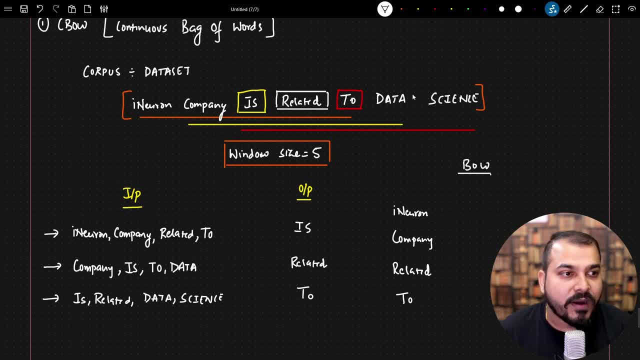 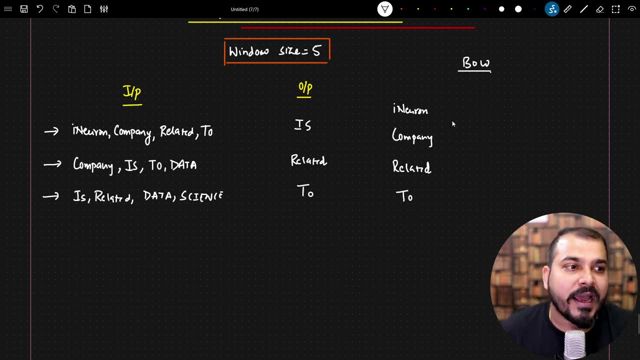 so over here you have one, two, three, four, five, six, seven, so seven total. unique vocabulary is there. now, wherever i have i neuron, wherever i have i neuron. what i'm actually going to do is that i'm just going to make it as one over here initially, and there will be six zeroes. so right, one, two, three, four, five, six zeros, right. 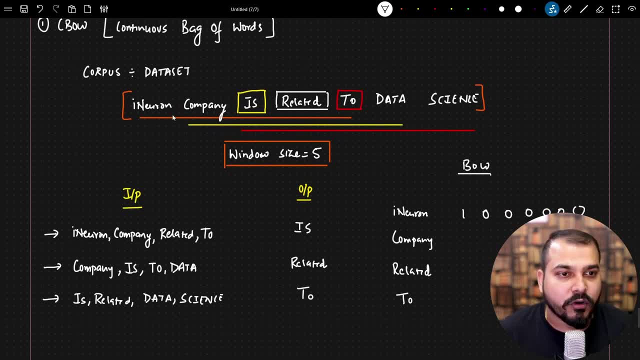 so, with respect to this entire vocabulary, wherever i have i neuron that will be represented as one: zero, zero, zero, zero, because remaining all the elements will be zero. right and now when i go to company company, what will happen then? my second element will basically have zero, zero, zero and all the 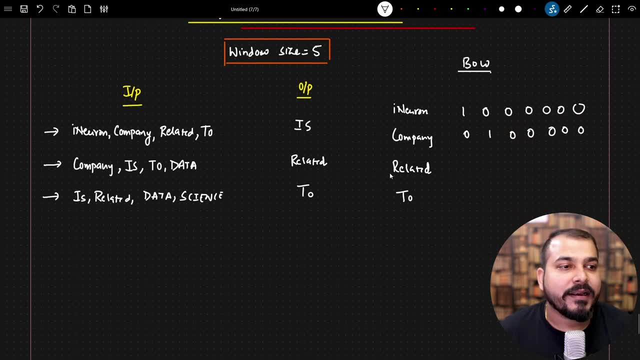 elements will be zero. similarly, if i have related right in related, which word will be zero? which world will be one, I go ahead and write it: 0 0 0, 1 0, 0, right, and finally, you'll be able to see that the next word 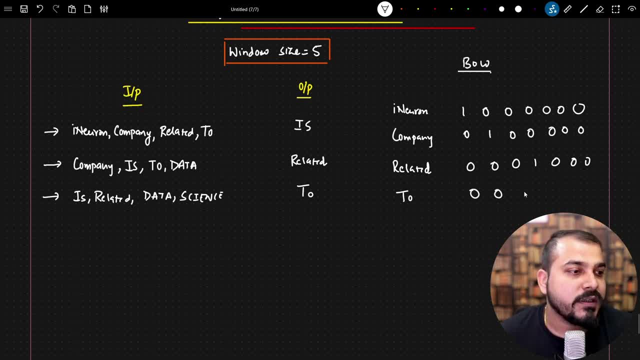 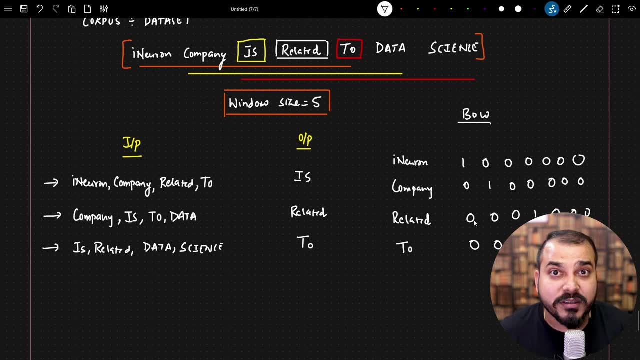 that I'm having is 2, so 2 with respect to 2. here you can see 0 0 0, 1 0, 0, right? so all these words are there, right, and this is based on the vocabulary size and this is what is my bag of word representation. 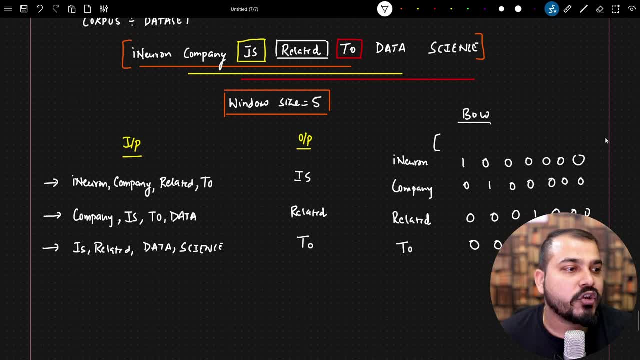 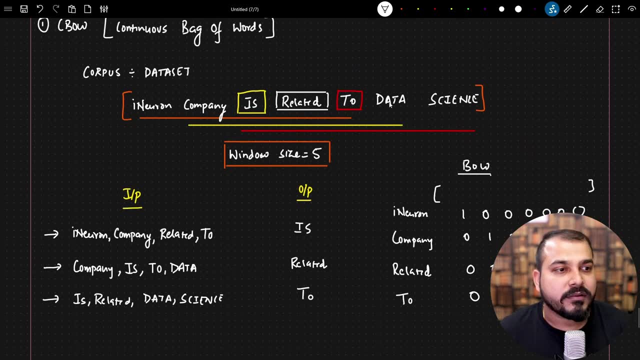 this. we have already learned it based on my, based on my vocabulary. what is my vocabulary? the first word is i- neuron, then company, then related to data science- right something? data science, right? so all these words are there. now, understand, this is what is my bag of word representation. so if I 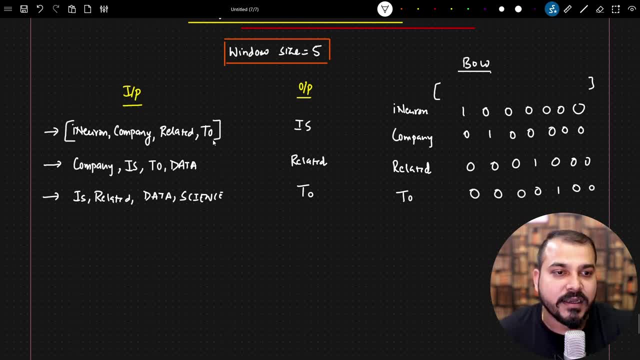 really want to represent this entire sentence. I basically need to convert this into this: dimensions right i? neuron will be given in this vector form, company will be given in this vector form, related will be given in this vector form, and 2 will be given in this vector form. very simple, right? every. 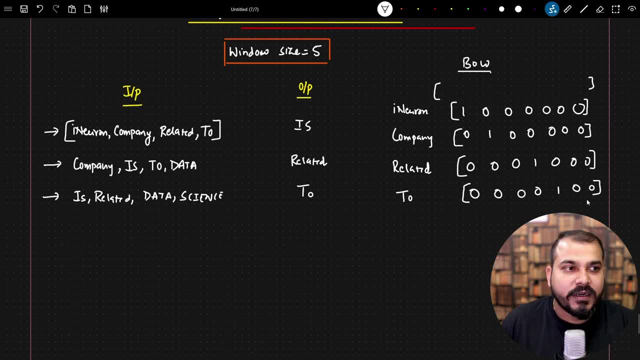 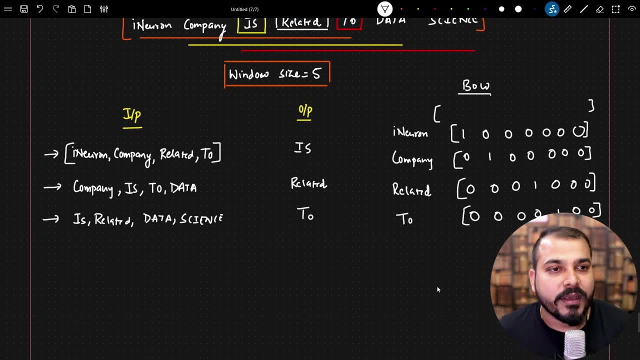 word is basically converted into a vector based on the vector size, right. very much clear, very much simple. I hope you are able to understand this right. so what I have actually done, based on the vocabulary side, I have actually converted each and every word into vector, wherever i neuron is there. 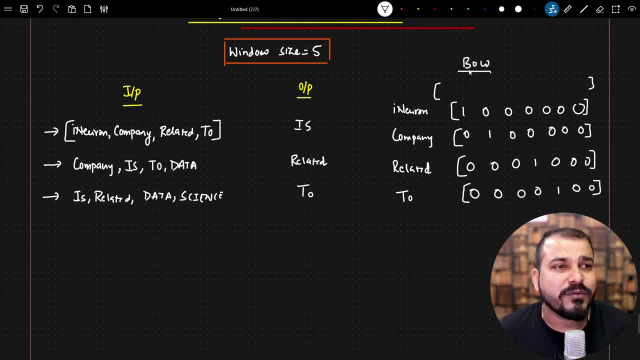 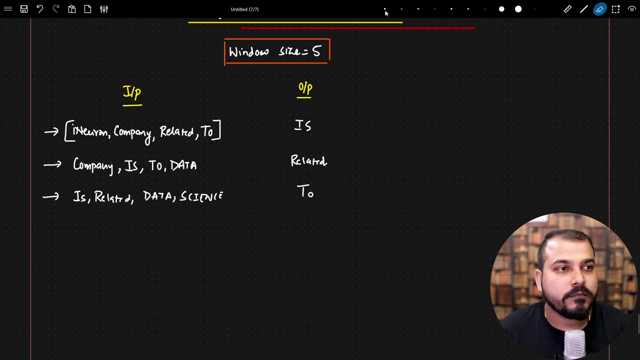 I'll not. I'll not say this as bag of words. I'll basically say this as one hot encoding right over here, as I understand this verse Now, one very important thing that you need to understand will be: you'll be seeing, i neuron company will be related to all these inputs and output. 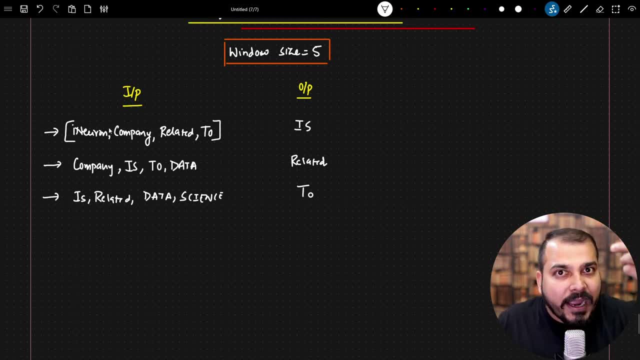 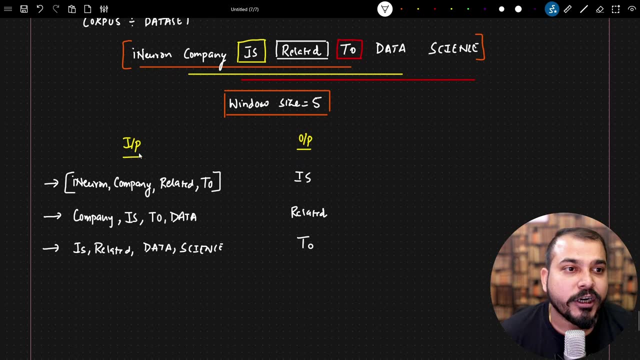 I cannot probably send the steps directly. I need to convert this to some vectors initially to send it in as an input to the neural network also. so this is what I'm actually going. First of all, you know that how many number of words i have. 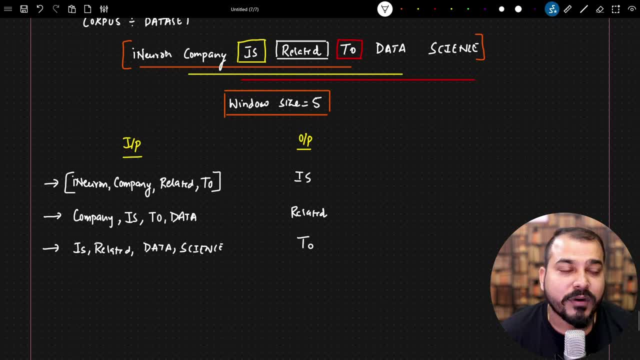 How many number of words i have in the vocabulary. i have i neuron and i게요 D Doctor directly i neuron. i have company i have is related to data science right. so they are on one, two, three, four, five, six, seven, right, seven words are there now, if i probably use one hot encoding technique. 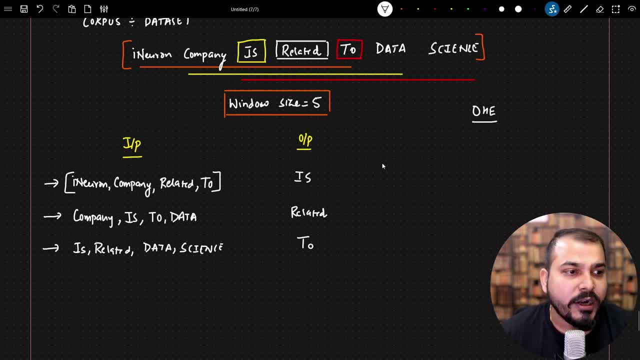 now see this. okay, this is super important in one hot encoding technique. if i probably consider i neuron, let's consider the first sentence over here. i have i neuron and then i have company, then i have related and then i have two right. so for all these words, how i'll be giving the one? 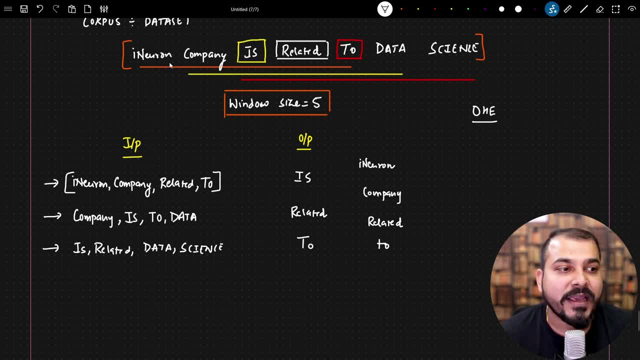 hot code, one hot encoding representation. wherever there will be i neuron, i'm just going to make it as one. remaining all will be zeros. so there will be around one, two, three, four, five, six zeros. similarly, when, when company is there, i'll make this as one and remaining all will be. 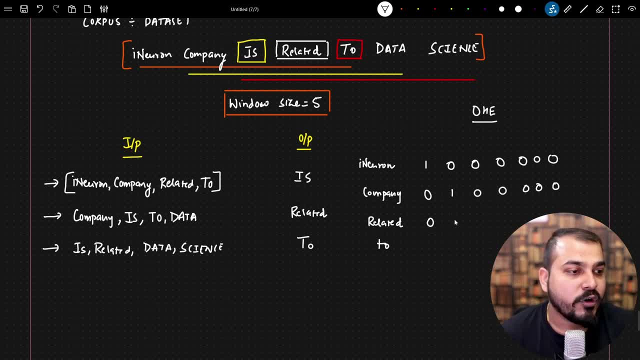 zeros, right? similarly related. related is in the fourth word, so i'm going to make it at zero, zero, one, zero, zero, zero, and then two is present after this, so i'm basically going to write it as zero one, zero, zero, right? so this is. this is pretty much clear till here, right? so here? 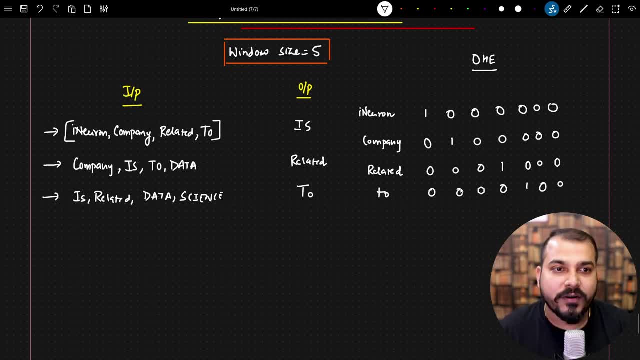 you can see that i have basically done this. a simple one, hot encoded format. that basically means if i really want to pass i neuron, i need to give this as my vector. this is what is the understanding, and this vector is basically given by seven dimensions. so seven vectors i'm giving. 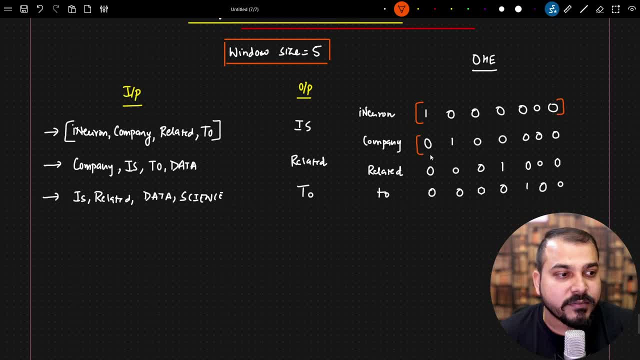 it over here, right. one, zero, zero, zero, zero. if i'm sending company as my next word, then this should be the vector it should go right. then if i'm sending related, this should be the vector i should go so. similarly, all these particular words will be converted into this particular vector using one hot encoding. 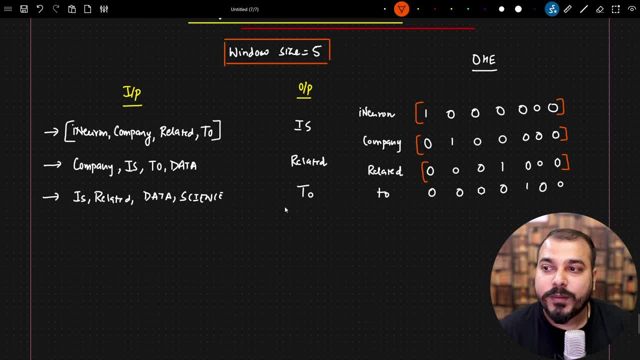 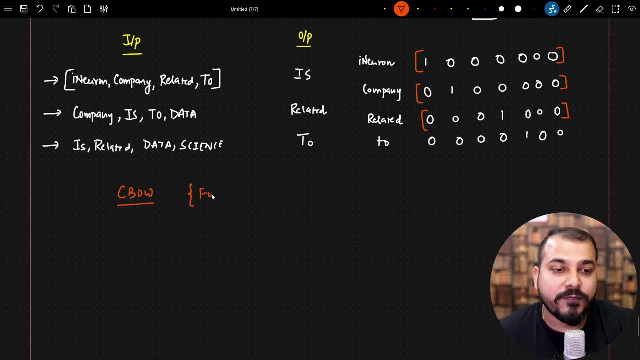 now let's go to the next step, which is super, super important. okay, super, super important. what does c bow basically mean? continuous bag of words. okay, this is nothing, but this is a fully connected neural network. now you will be able to understand how this models are created. fully connected neural network. okay, now in this fully connected neural network. 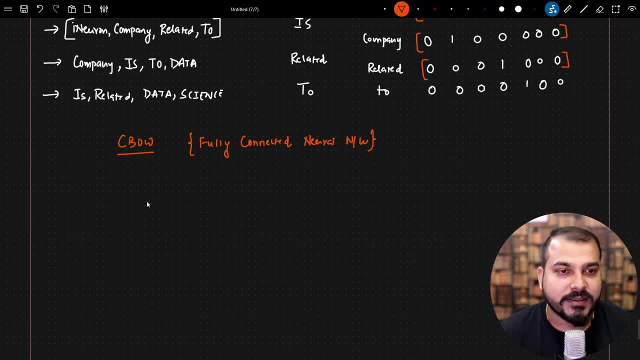 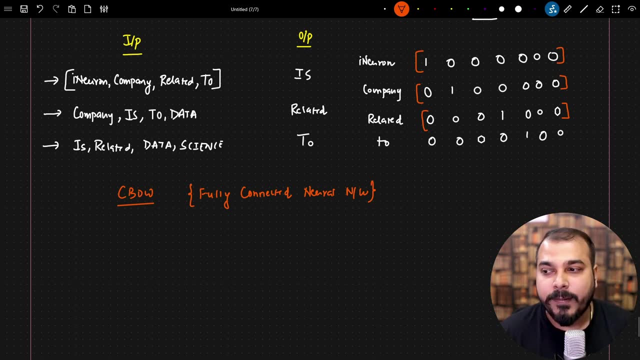 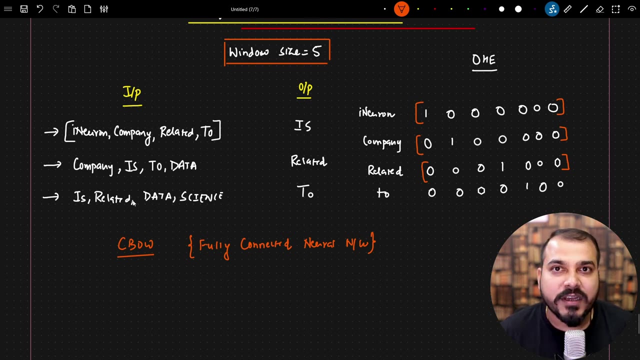 you will be able to see one very, very important thing. one is, first of all, just understand how many number of input should i be giving right, like how many words i will be giving as my input right? since my window size is same. window size is five. all my inputs are fixed. i hope that is very. 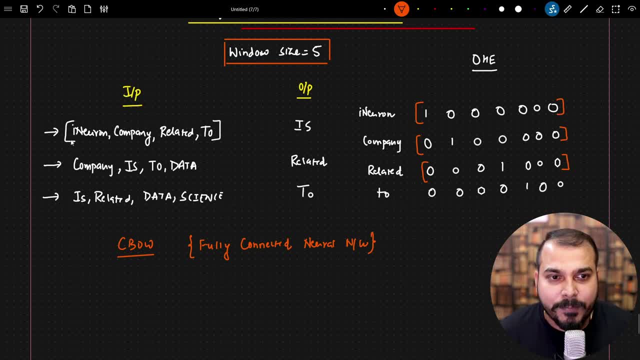 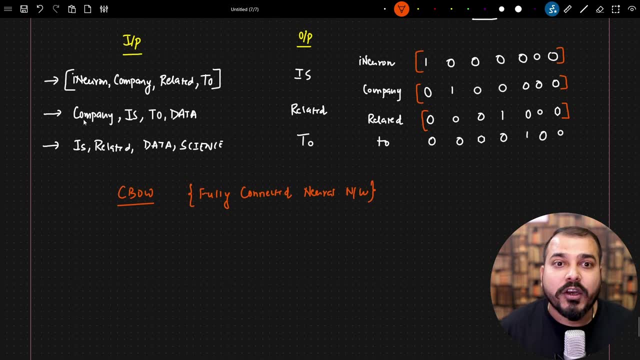 much clear right now. in this particular problem statement you'll be seeing i'm giving four words in every sentence, so my input is basically fixed. now i neuron. when i give my word, i neuron. let's say, in the first case i give my sentence one and this is my sentence one. when i give i neuron, i neuron is. 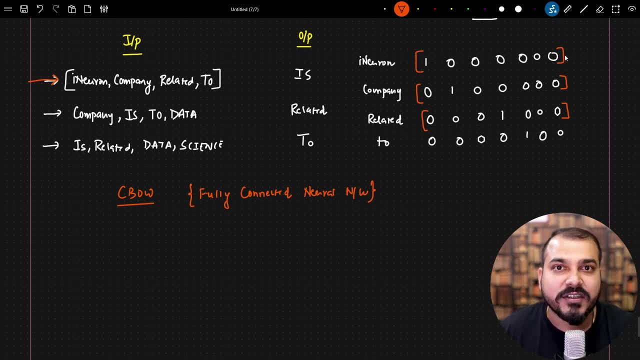 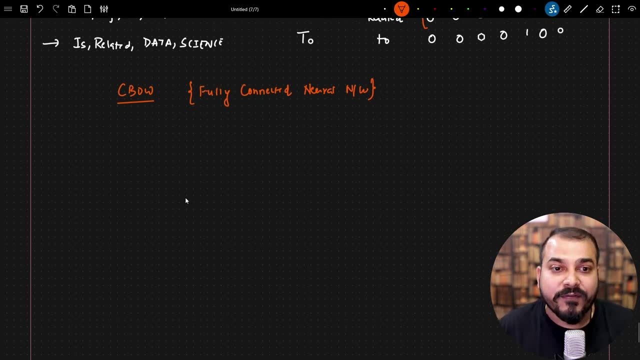 represented by seven vectors over here it is represented by this vector, then company is basically represented by this vector. so if i probably see in fully connected layer, my first input layer will basically be nothing, but so here you will be able to see this will be my input, okay. 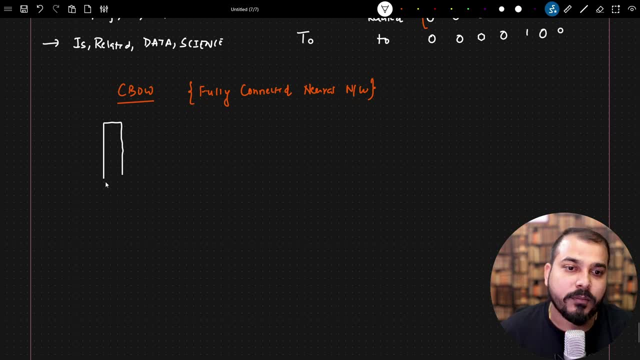 i see this. so this will be my input, my first input word: okay and understand, i'm giving, i'm creating this circle as my inputs. okay, i'm, i'm just creating this circle as my input. so if you see one, two, three, four, five, six, seven, seven inputs, i'm giving it right now, when i give this seven inputs, then 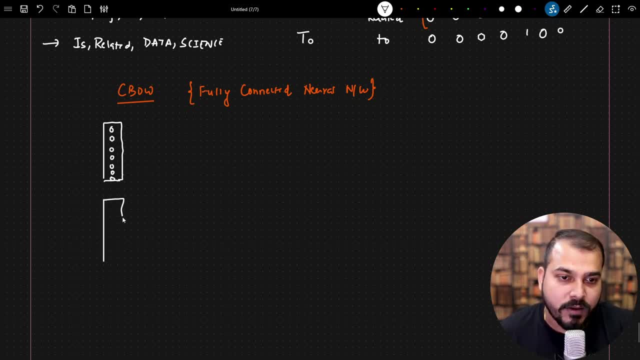 similarly, how many words will be going? four words will be going right. so one word, two word. so this is input layer. so this layer is nothing but my input layer in a fully connected layer. a simple a and n, if i probably consider an example of a and n. so here also how many inputs i'll be having: one, two. 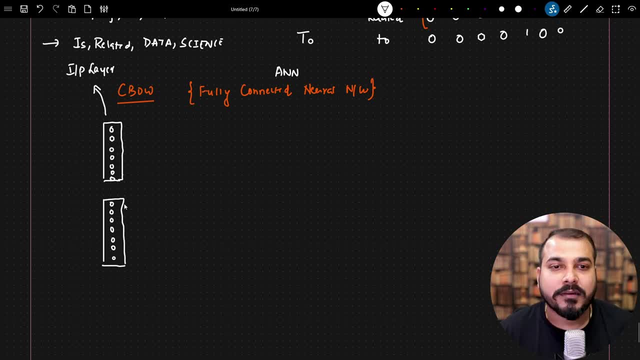 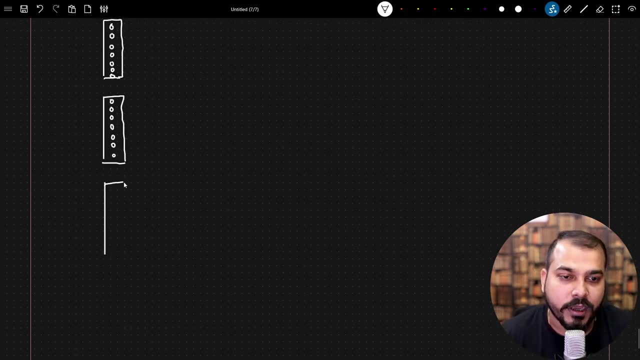 three, four, five, six, seven, right- and this is my first word- second word, third word, fourth word. so i will be having four different words over here that will be going and each word will be having a dimension of seven vectors: one, two, three, four, five, six, seven, right. i'm not giving this value. 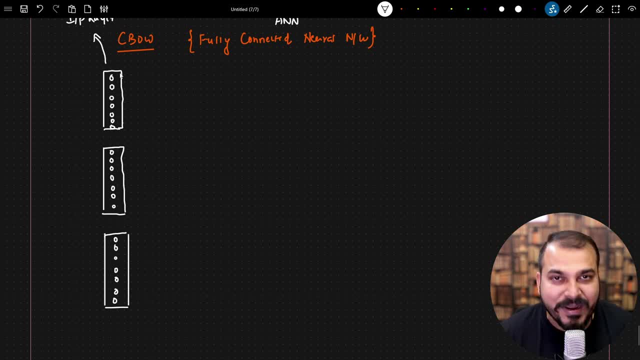 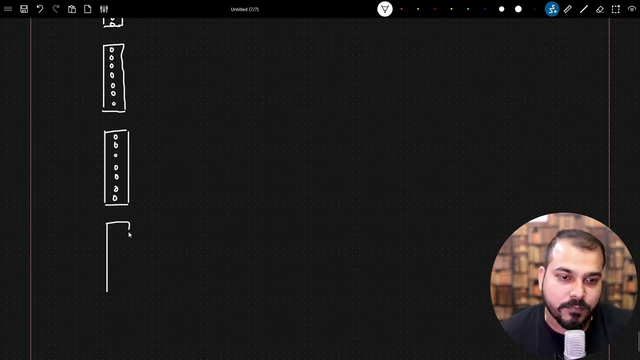 don't consider that these all are zeros. okay, i'm just saying that these are my input layer, input layer, input circles. okay, that is how we create it in a and n, right, and then probably i have my last one. so this is my input, right? i'm basically designing the neural network, how it will look. 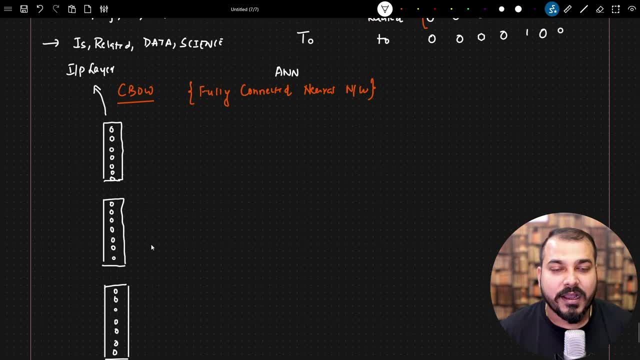 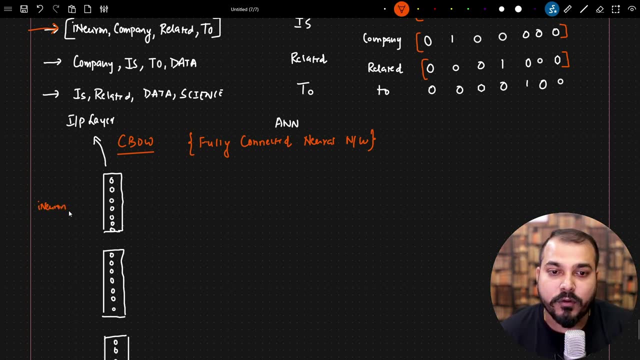 like when we are training a word to work. so these are my four, four words, understand. in the first case i'm going to pass i neuron over here. you. so let's say i'm going to pass over here i neuron. this will be my input over here. this is represented. 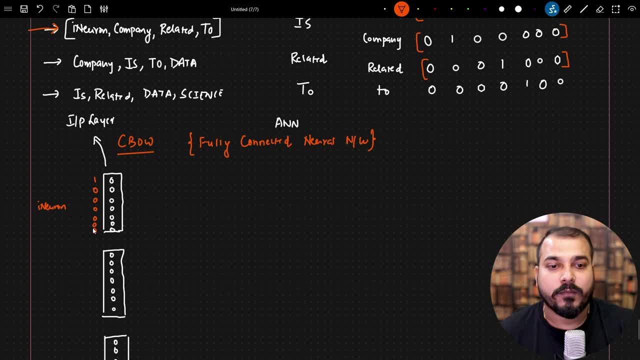 i neuron will be represented by one zero, zero, zero, zero, zero, right. and similarly, if i go to the second word that is like company, then it will be represented by another word, like this: right. it will be represented by a different vector, like zero, one zero, zero, zero, zero, zero, right, seven. 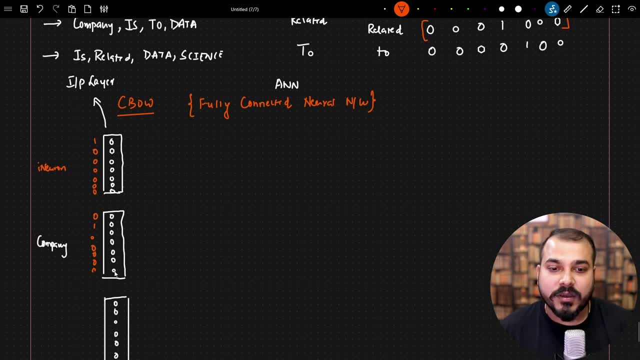 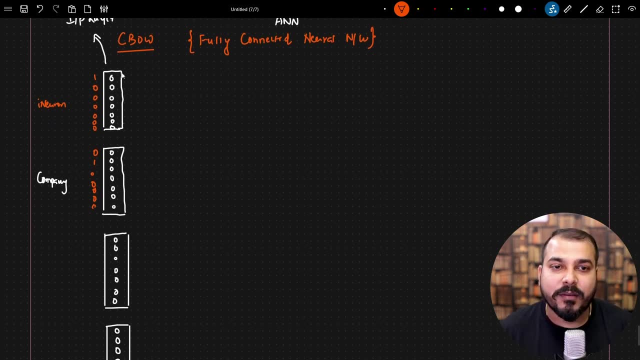 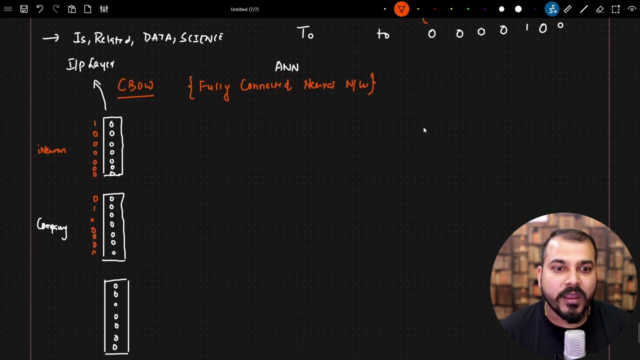 it will be one, two, three, four, five, six, seven, right now. similarly, other words will be represented like this: okay, so this becomes my the input layer. okay, and every input is basically given by a vector of seven, seven dimensions. so, because i'm representing every word based on the vocabulary size using one hot encoder, now this: 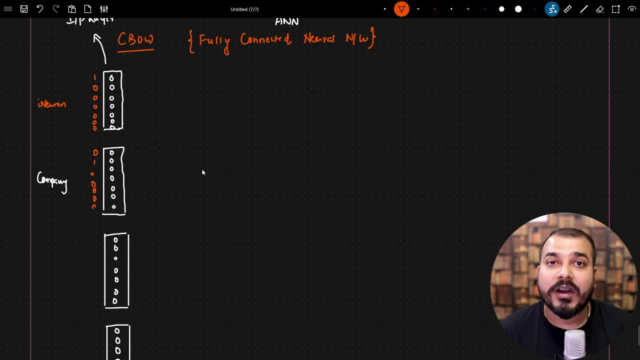 becomes my input layer. now let's go to the middle layer. that is called as a hidden layer. now, in this hidden layer, this is super important. just pause the video and guess what will be the size. you know the our window size is how much. our window size is basically five, right, so i'm just going to make 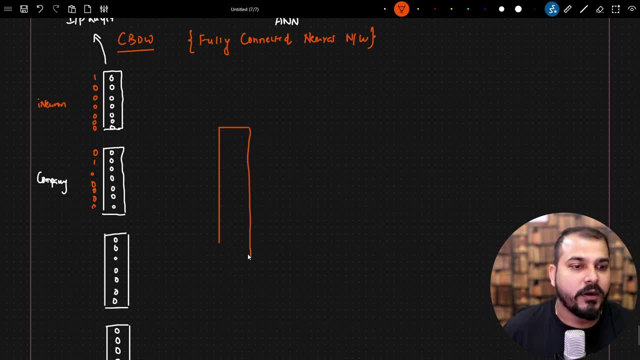 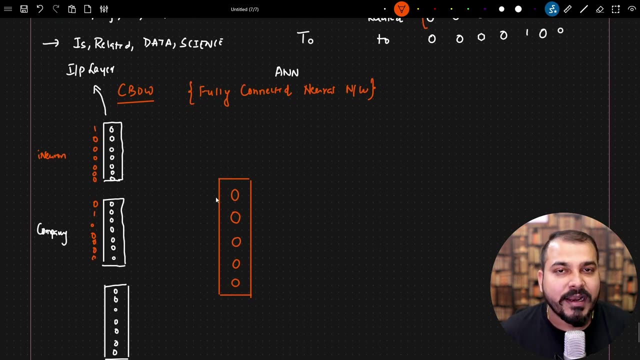 this as my window size. okay, so this is my window size. now in my window size, if you remember how many, how many we are having in our window size, our window size is nothing but five, so i'll be having one, two, three, four, five. right window size is basically five, so in my hidden layer i'll be having this: five vectors. 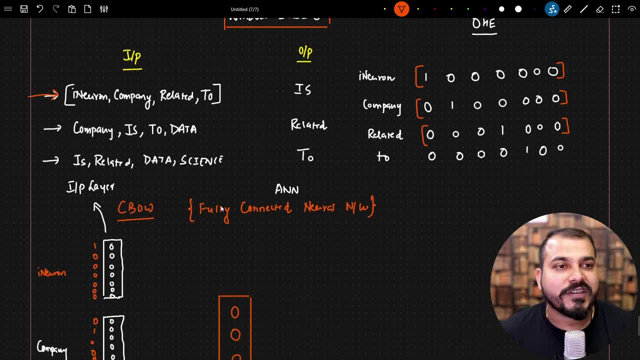 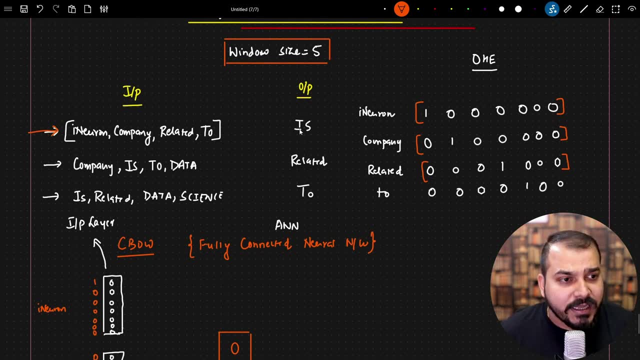 okay, so just understand that, with respect to this five, our window size will be set over here. okay, now, with respect to the output. in output, how many values i have? i just have one value and each word. i just have one word in the output, right, and each word is represented by a vector of seven. 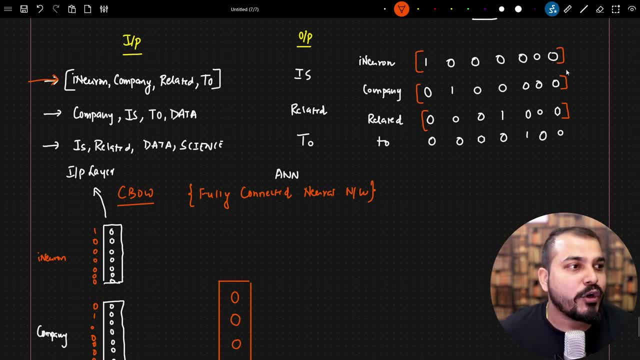 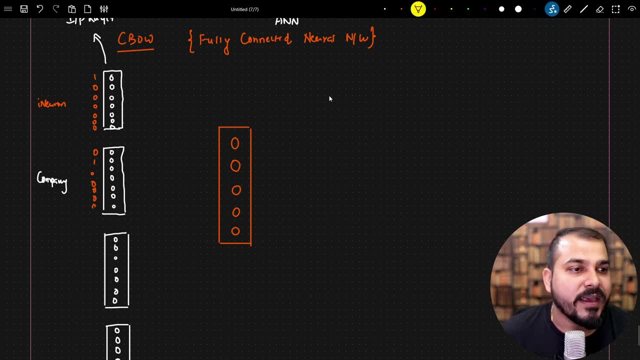 because if i am also considering this is using one hot encoder and i'm going to get this vectors of this dimension, that is seven, right? so what i will be doing in output, i will basically be having another output layer like this, which will again be having seven different outputs. 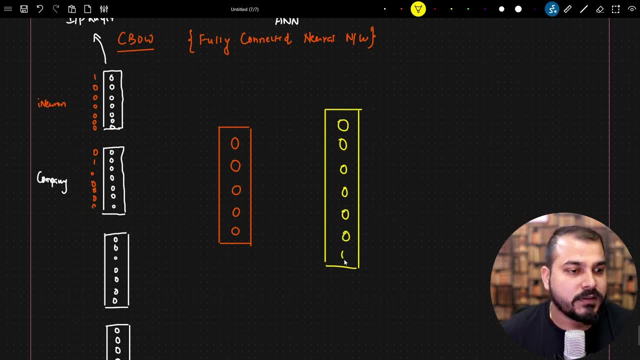 one, two, three, four, five, six, seven. okay, now this is how my fully connected neural will look like. neural network will look like. now. you need to understand one thing over here: each and every node, each and every node, will be connected to the other node, right like this. 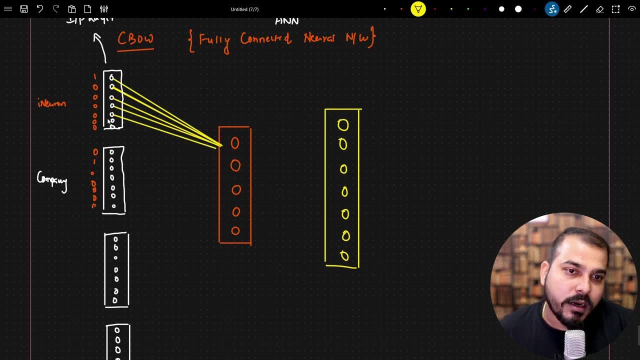 like this. it will be connected like, like how an ann will work will be connected like this, only right. similarly, right now, similarly, these all will be connected to this also. so, in short, i can basically make a very simple connection like this, which will look like this itself, and this will be entirely. 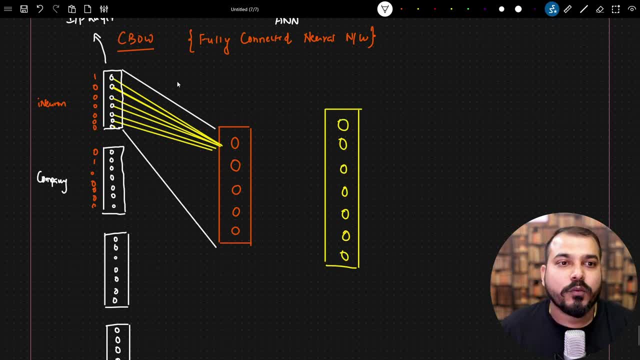 connected to this right. understand, all these lines will have some initialized weight, initialized weights, and we need to train these weights and this is what it happens in ann right. similarly, this will be connected to this, this will be connected to this, this will be connected to this and, finally, this will also be connected to this. 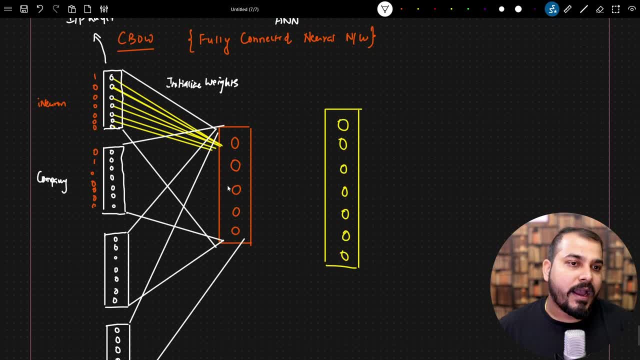 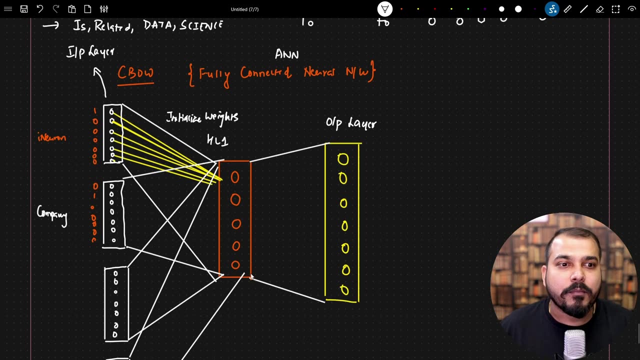 right, so everything is basically getting connected, and from the hidden layer- this is my hidden layer one, hl1, and this is my output layer right now- from this hidden layer it will basically get connected over here and this will get connected over here. okay, now understand one very, very important thing. 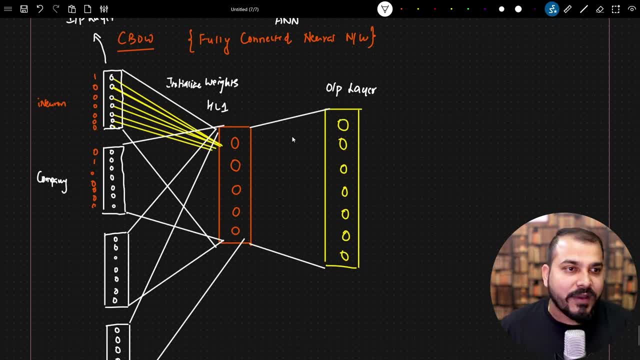 okay, this is super, super important. fine, we are connecting it with the help of loss function. we'll also do forward and backward propagation. now let's say we'll consider, let's, let's pass this particular word: i neuron company related to. so i have passed i neuron company and here also you'll 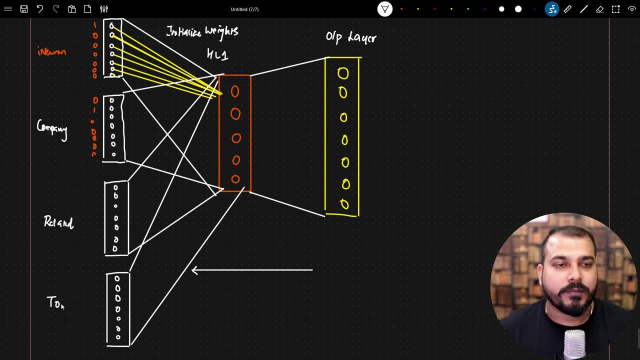 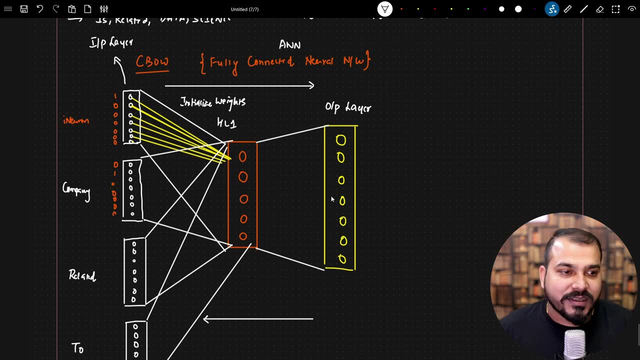 be able to see i'm passing related to very simple. okay, let me just zoom out a bit. okay, now, once i pass all these things, what happens over here with respect to this 7 output? i already know what is my real. output is right, i'll be getting some values over here. okay, i'll be getting some values, okay, but 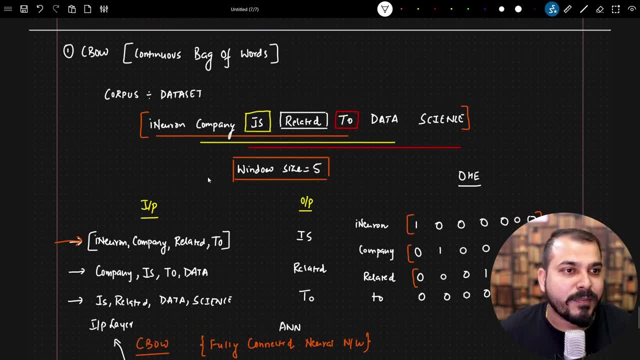 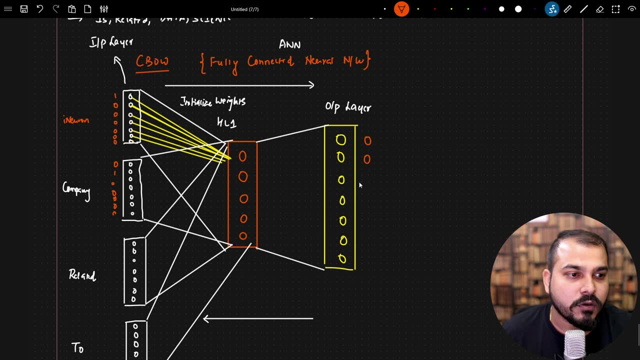 the real output is what, if i consider is? is is my third word, so is is my real output. so this will basically be represented in this vector format. that is zero, zero, one, zero, zero, zero, zero, right. but after training, while we are training the model with different, different weights, this is my true. 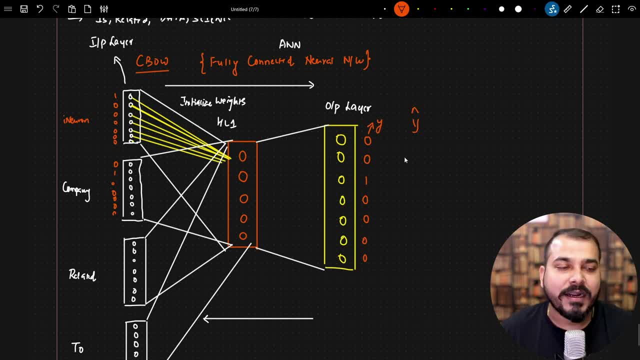 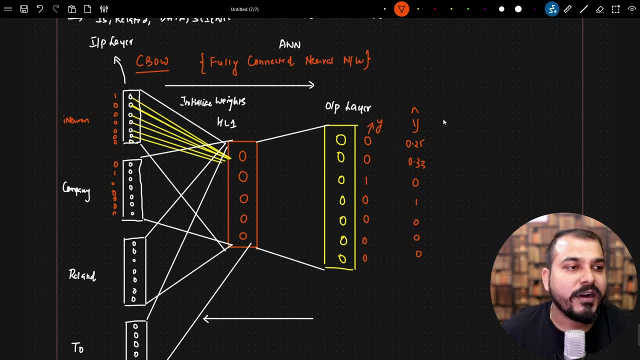 0, 1, 0, 0, 0, something like this. then what we do? we basically calculate the loss function and, based on this loss, we need to reduce this. we do the backward propagation- right backward propagation- and we do it unless and until the difference between y and y hat are minimal, okay, and this process is continuous. 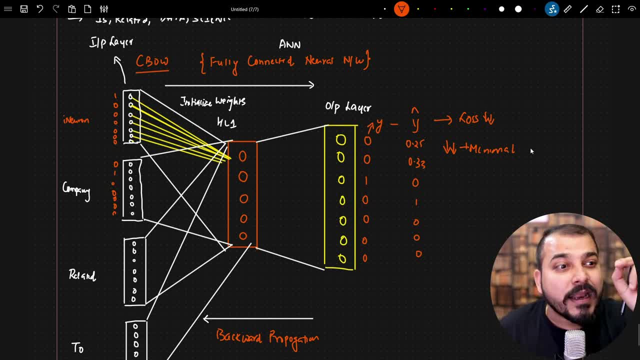 very simple, but now you nearly need to understand one very important thing, very, very important thing now, since this is giving me a specific output. okay, this is basically giving me a specific output when i say my, my middle layer is basically window size of five, window size of five. that, basically. 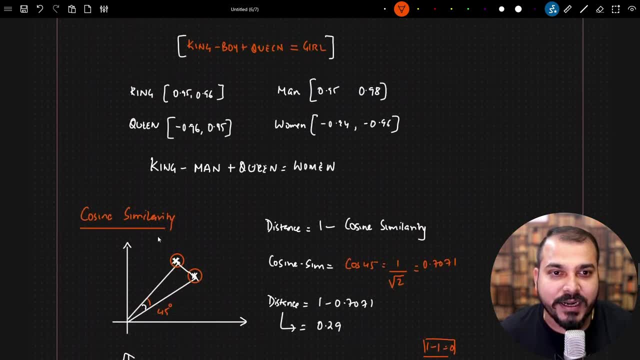 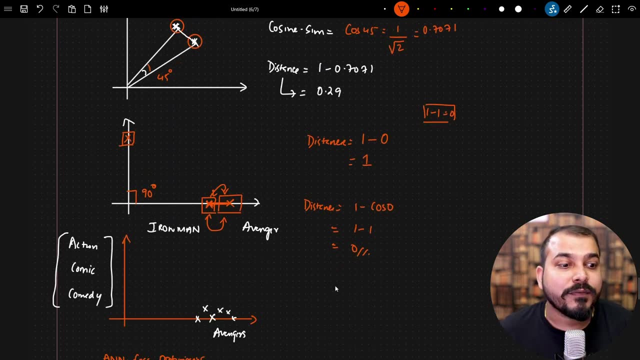 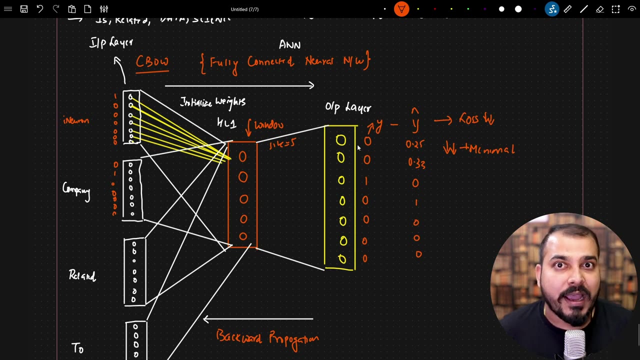 means over here in the word2vec. when i said i will be getting a 300 dimensions over here when i'm using google word2vec, this is all because of this window size. okay, that basically means if my window size is five, i'm going to get the output as five for every word. that basically means when a word is getting. 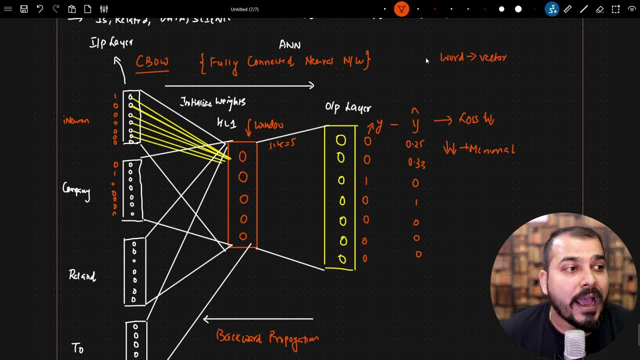 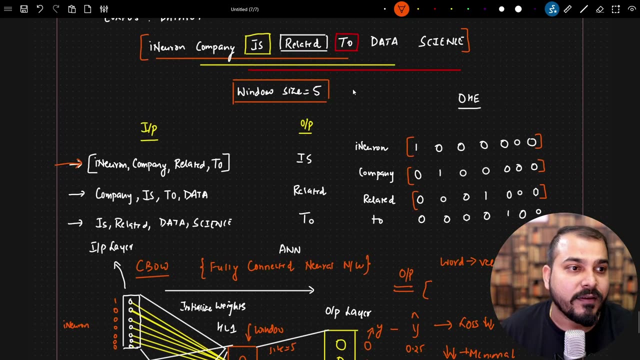 converted into a vector. i am going to get a size of five vectors and this will be basically be my final output now. i hope you are able to understand again. let me repeat it: the reason i have actually selected window size is equal to 5 because i want to probably provide a feature representation. 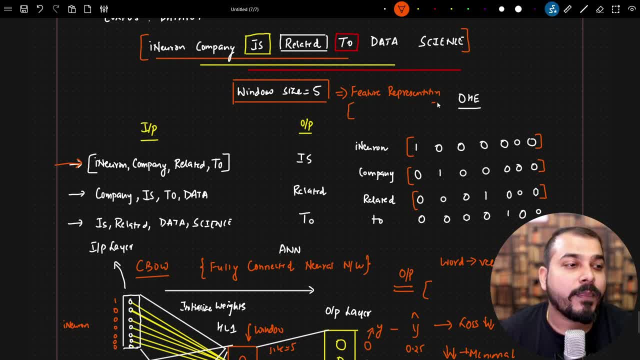 over here. in the model of window size. that basically means if i select a vector size of 5, okay, that basically means every word will be converted into a five vector. now, when i took an example of google, which was getting converted into 300 dimension, that basically means my window size. 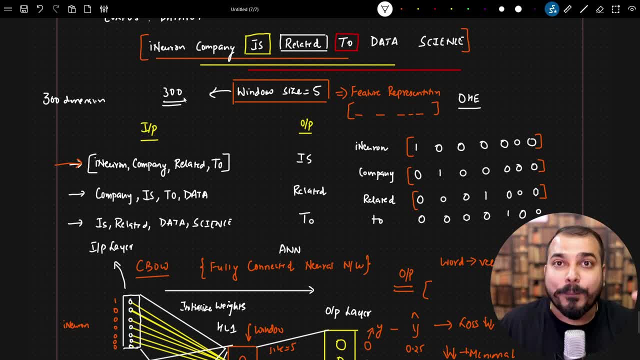 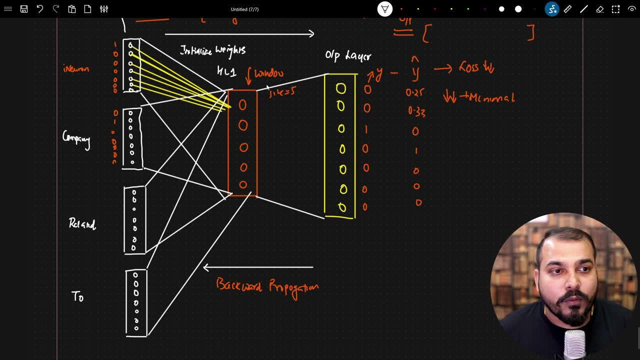 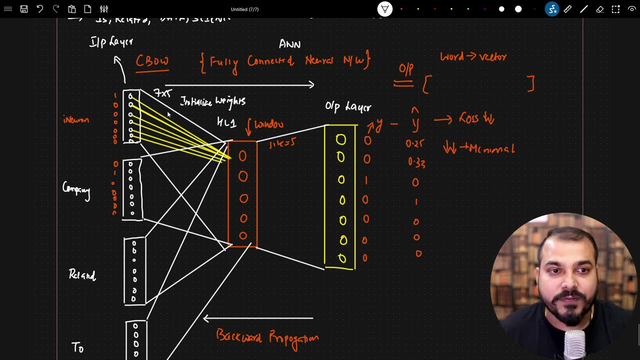 is 300 and more. the bigger window size, the better the model can basically perform. okay, so in this case you'll be able to see that over here. my window size is five. that basically means if i see from starting right, My matrix for every word will be 7 cross 5.. That many number of weights. 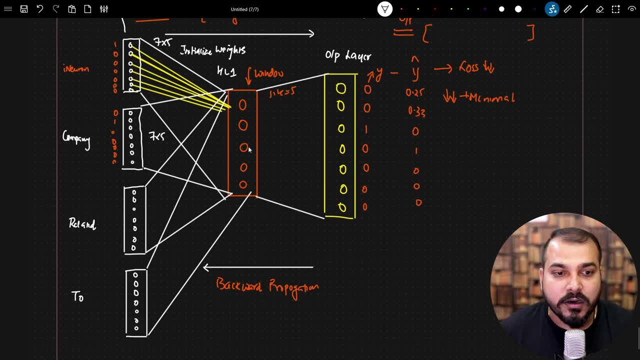 will be there. Then here also I'll be having 7 cross 5 weights. Here also I'll be having 7 cross 5 weights, because I'm giving 7 different vectors. Here also I'm having 7 cross 5.. But in this case, 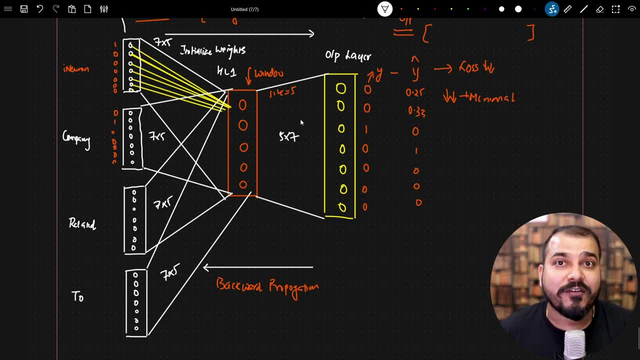 I will basically be having 5 cross 7.. Now, what does 5 cross 7 basically mean? When this loss gets reduced, then my final vector will look something like this: This all will get connected to this. This all will get connected to this. Let's say, it is getting connected to this one. 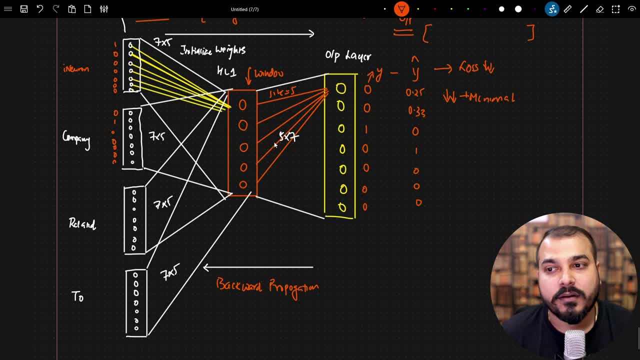 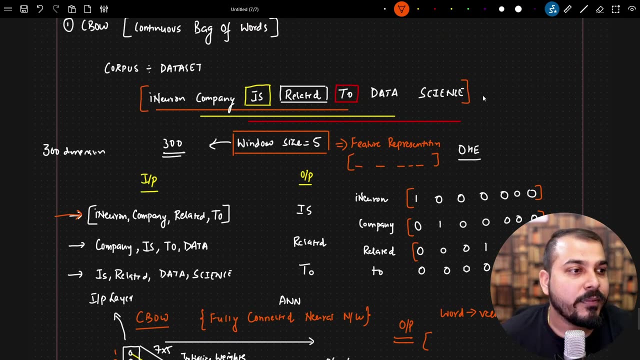 It is getting connected to this one. It is getting connected to this one. So, once we have this particular connection, let's say our first word over here is: what is our first word? If you probably see what is our first word with respect to this particular vectors, with vocabulary, We'll 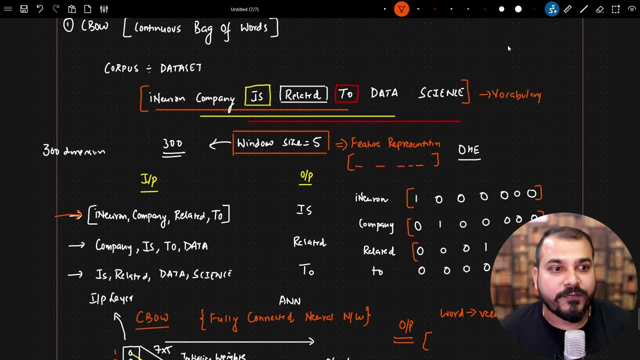 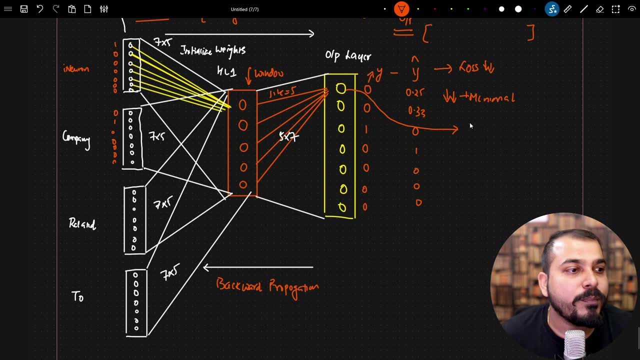 be seeing I neuron. right, This is my vocabulary. The first word that is basically getting represented over here is I neuron. So I neuron will have an output dimension of 5 vectors, because I'm getting these 5 vectors over here joined to this, So these 5 vectors will be like 0.92, it can be 0.94.. Based on the training, 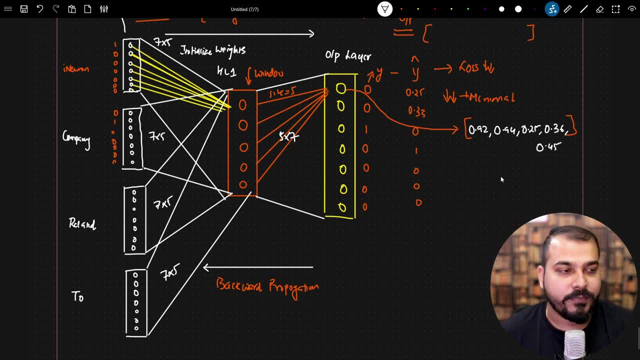 it can be 0.25, it can be 0.36 and it can be 0.45. And this is based on some feature representation. So I hope you are able to understand and this is how I neuron will be represented. 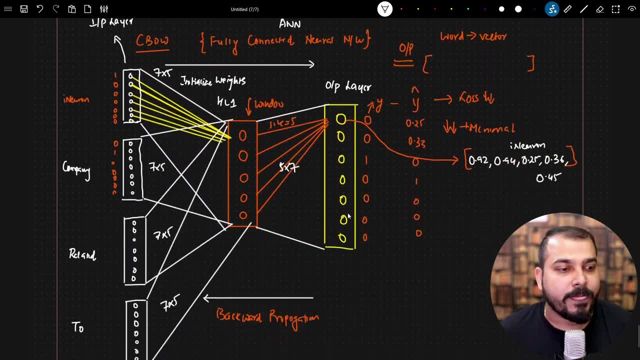 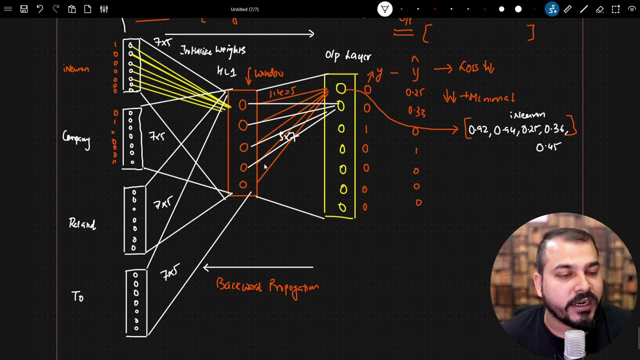 the second word that we have in the vocabulary, that is, company. right, this will again get connected to this company. this will also get connected. this will also get connected. this will also get connected. this will also get, and this entire word will be the vector for the company itself and for the company we.